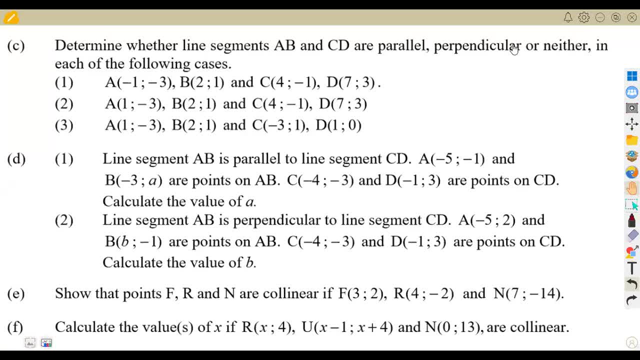 Hello guys, welcome back to Maths on African Motives. We are still on our mathematics. for Britain This is analytical geometry. as we are having a revision actually on our gradients, We want to have a continuation to check more about the gradient concept. What is it exactly? 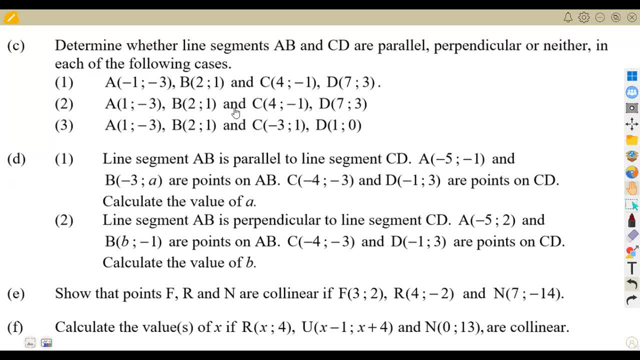 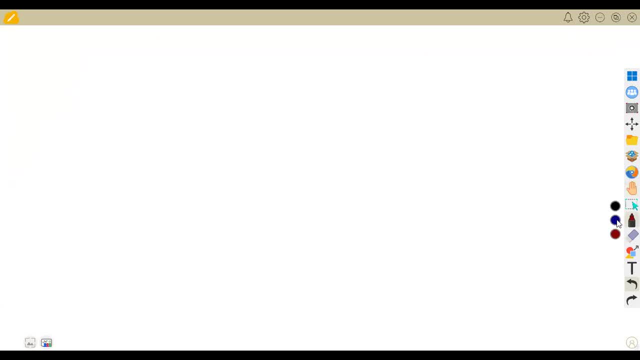 that we are talking about on this gradient and how is related, like I said from the previous class that we had, that we shall have a continuation whereby now we shall be talking about the issue of parallel lines, perpendicular lines being collinear, this and that Okay. 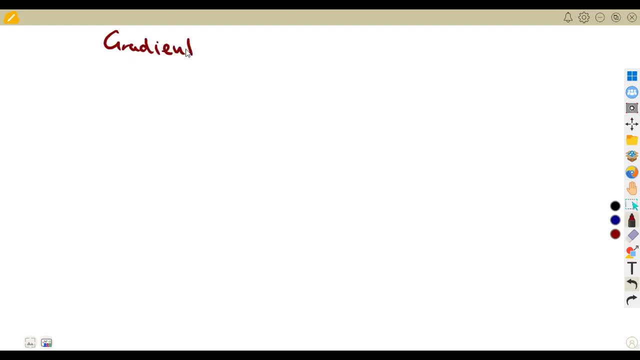 so we are still on the gradients, on our analytical geometry, working with the gradient. So remember from our previous class that we had, I say the gradient can be taken as from two points. Okay, if you take the gradient from two points, being the change in y. 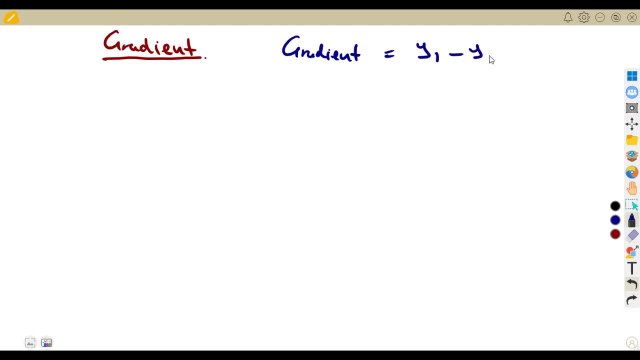 over the change in x, and last time we used y1 minus y2.. So I do not want to confuse you. So I'm just going to use this formula so that, so that we can have what? the same thing throughout, but it can be written as y2 minus y1 over x2 minus x1, like I said in our previous class. 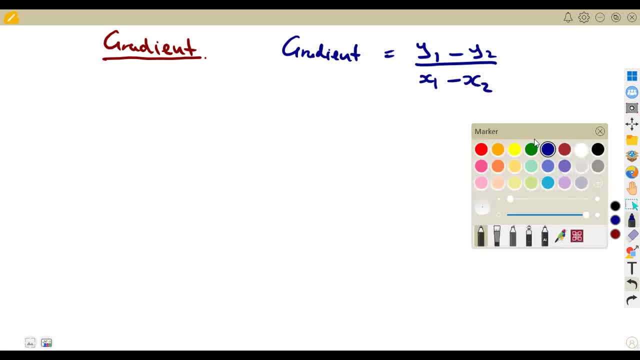 The concept that we had on that gradient and I said you can also use the letter m to represent the gradient. All right, in short, you can just use the letter m to represent what we call the gradient. So it follows that. let's say I have got two lines. 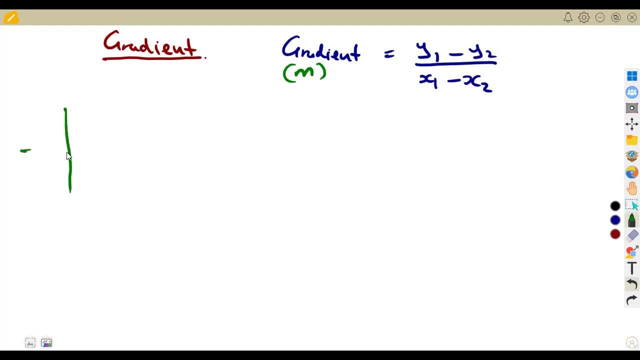 that are parallel. Okay, remember the concept of our Cartesian plane. we talked about this, that for the x and y on our Cartesian plane, this is a line. y is equal to y is equal to this. These are two lines That are parallel. Remember, two lines that are parallel means that they have got equal distance. 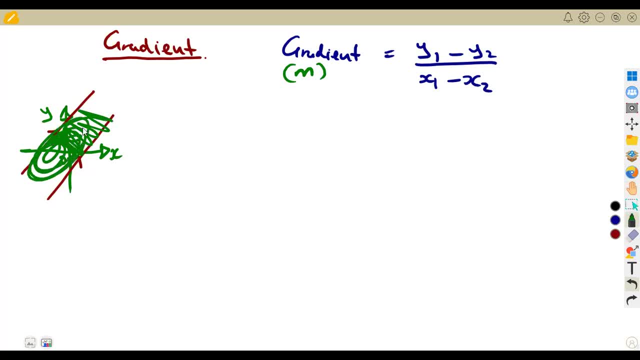 in between. They do not meet. these two lines that we see here They do not meet, That is to say, these lines, they are parallel. So let's say this is the first line and this is our second line. It follows that the gradient of the first line right as long. we are dealing with what parallel? 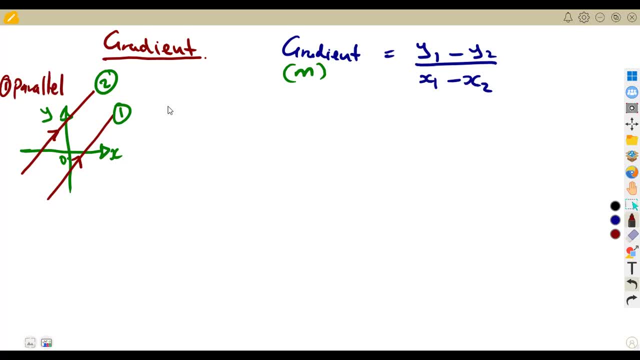 lines. So this is for parallel lines. So it follows that as long we are dealing with these parallel lines, they have got equal gradients. And I said gradient can be written in terms of m. So if we are saying that parallel lines, they have got same or equal, they have got same or equal, same or equal gradients. 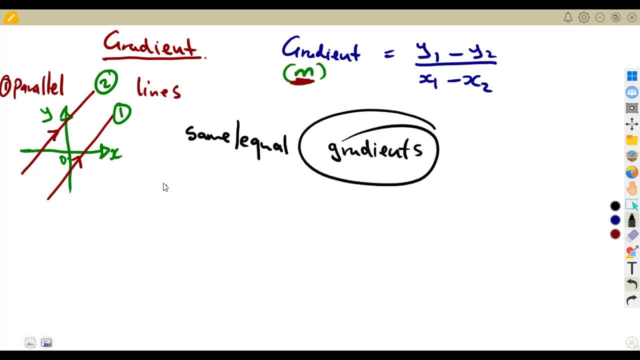 So these two lines, they have got same gradients. All right, The gradient of the first line and the gradient of the second line is the same. So if the gradient of the first line and the gradient of the second line are the same, or the gradient, 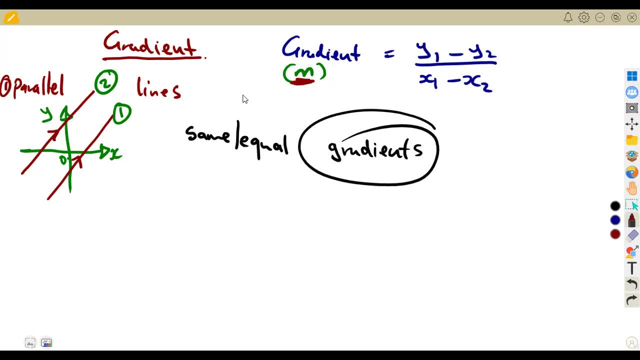 of the first line and the gradient of the second line are equal. what does it mean in terms of simplification in an easier way, We say: the gradient is m, So it follows that we're going to have m1 for first line is equal to m2 for the what, The second line? Because 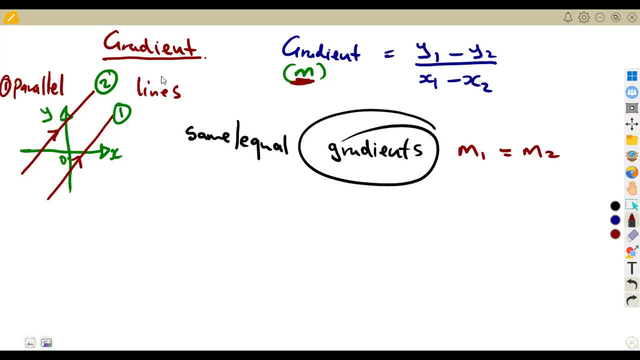 we're talking about two lines That you are comparing to. You are comparing the gradient of two lines that are parallel, Two lines. So you're going to have line one and line two. They are parallel, They have same gradient. m1 must be equal to m2.. The gradient of the first line must be equal to. 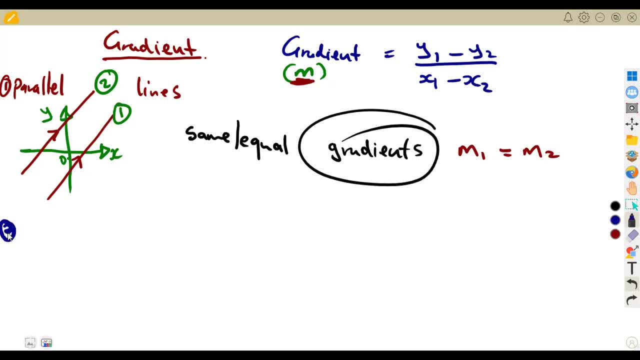 the gradient of the second line. Okay, What if these two lines are perpendicular? We can write an R and R condition of perpendicular lines. What are perpendicular lines? Yes, they are on the Cartesian plane, We know that. Okay, They are on the Cartesian plane, But 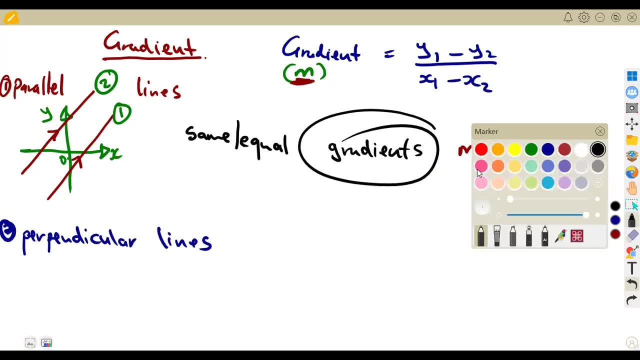 okay, The other thing, before we talk about this, the symbol that we use for parallel lines. Okay, So maybe AB is, maybe I want to write that AB is parallel. AB is parallel to CD, like this: I want to write this statement in short: AB is parallel to CD. I can write this as AB. 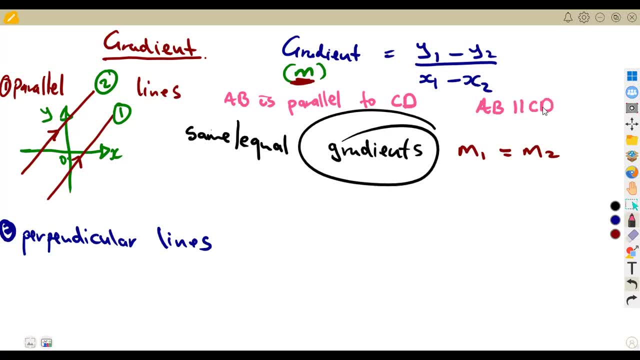 is parallel to, like this to CD. So this is the symbol, These two lines that are up. They show that it's parallel to. Okay, If they are perpendicular, I want to write in short that AB is perpendicular. Okay, AB is perpendicular to. AB is perpendicular to CD. All right, Let's say this time: AB and 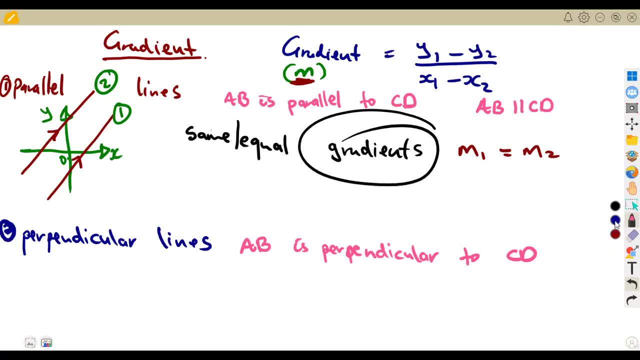 CD. They are perpendicular. All right, I can write this in short: AB is perpendicular. I'm going to use this sign for perpendicular- This sign is for perpendicular- to show that there are two lines which meet. at what? At 90 degrees. So that is what we're going to. 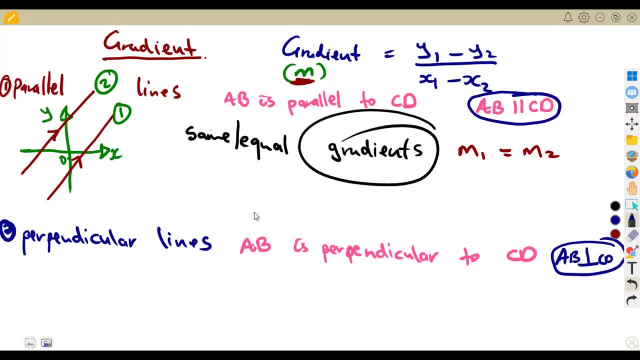 you're going to have for the parallel. we're going to have this, okay, but our idea is not about this symbol, and so our idea is: what is the relationship that happens for the two lines that are perpendicular? we've got two lines which meet at 90 degrees. all right, the first line, uh, and the second. 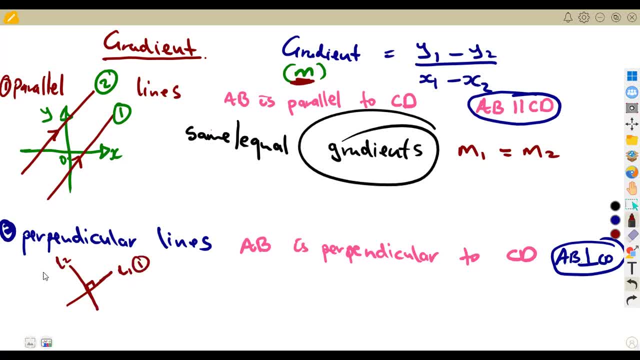 line that you're gonna have. so let's say, this is the first line that we have and this is the second line that there also, it is going to be compared in terms of their gradients to check whether a line is parallel or perpendicular. we use the gradient. so what is it about this? if they are perpendicular? 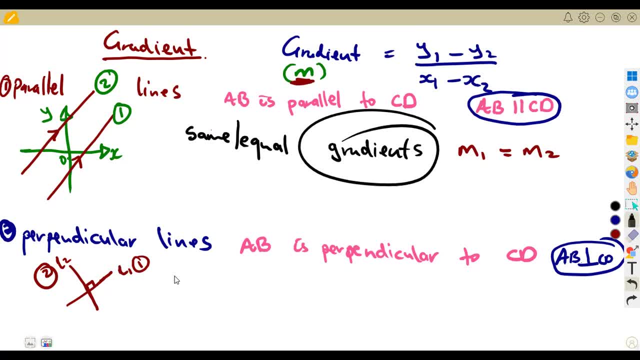 it follows that the product of these gradients is equal to one negative one. so, for perpendicular lines, for perpendicular uh lines or for perpendicular lines, uh, the product, all right, the product of the gradients, the product of the gradients in that case. all right, gonna talk about the product. 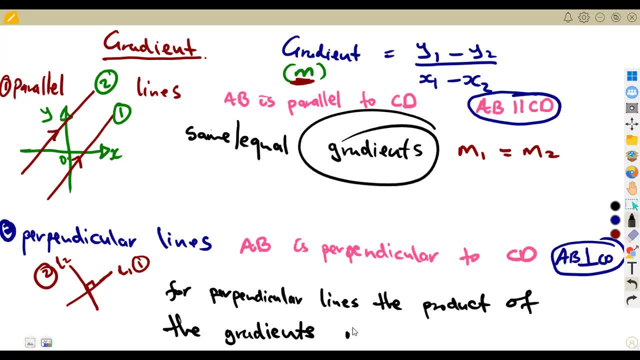 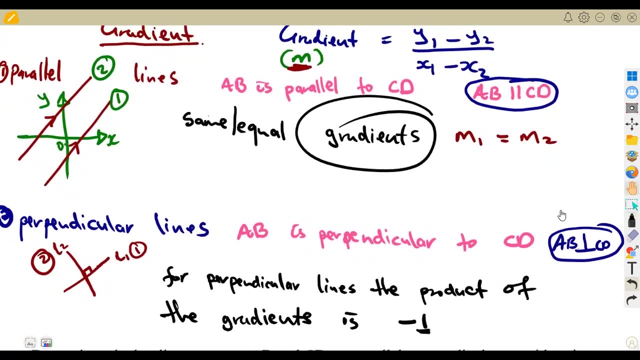 that is going to happen on the gradient is a negative one. this is what we have for perpendicular lines. the product of the gradients is negative one. what, what? how can we just write this in short, just like this, m1 is equal to m2, so it follows that, suppose. 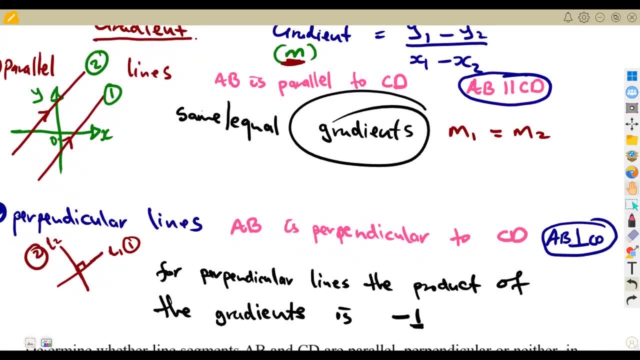 you're talking about the product, and this is the gradient of the first line and the gradient of the second line. so it follows that m1, representing the gradient of the first line, times m2, representing the gradient of the second line, is equal to negative one. So 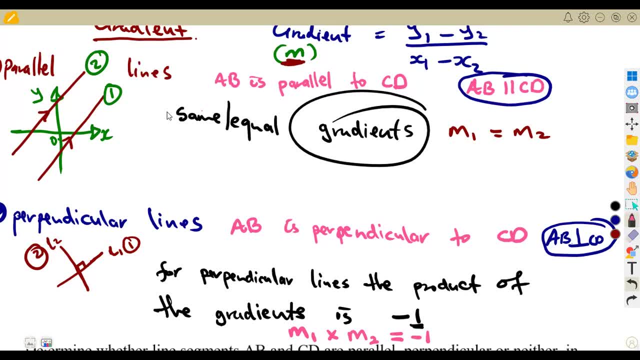 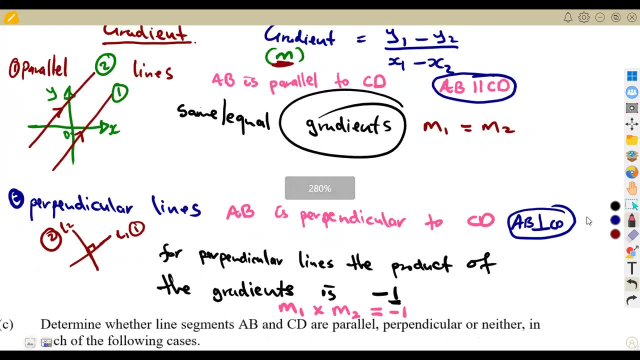 this can help us to determine the gradient of the other, or to check if two lines are perpendicular to each other, or to determine the gradient of the other line, given the garden of the other line and we are given that these two lines, they are perpendicular to each other. we 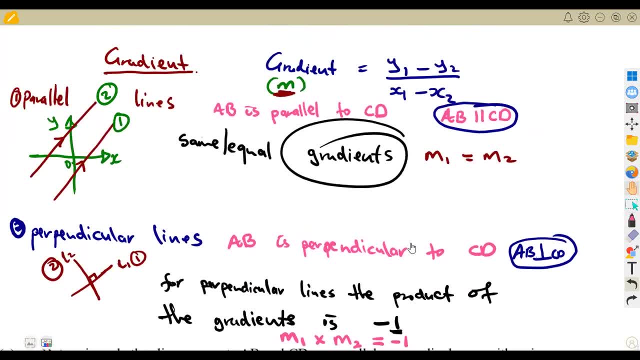 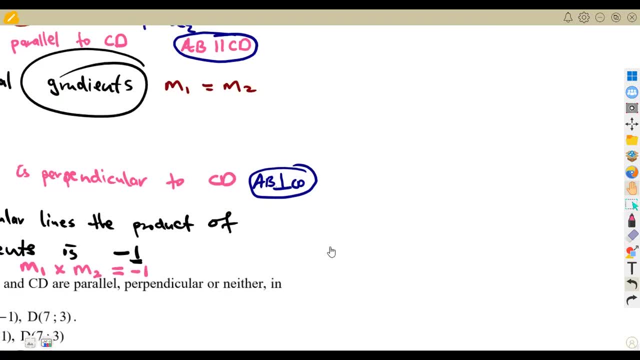 can use that as an advantage to calculate even the gradient of the other line. all right, then the last part that you're gonna have is when these lines are for linear. all right, so for the idea, uh, or we've got the scenario that we're gonna talk about core linear, all right, so this is core linear. 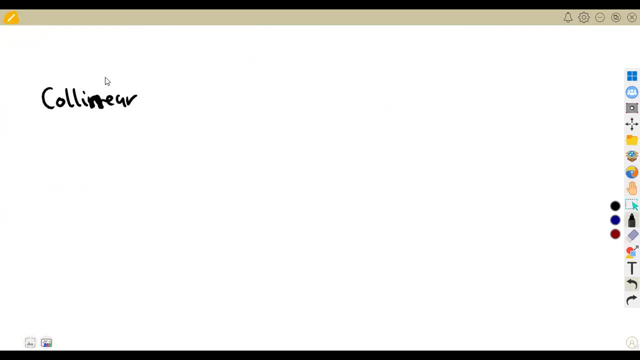 so for the core linear concept, we are simply saying we have got two things that we can consider. uh, in fact we are considering a straight line. we are still on a straight line. that is where we are. but now consider that there are three points there. okay, just for an example, there are three. 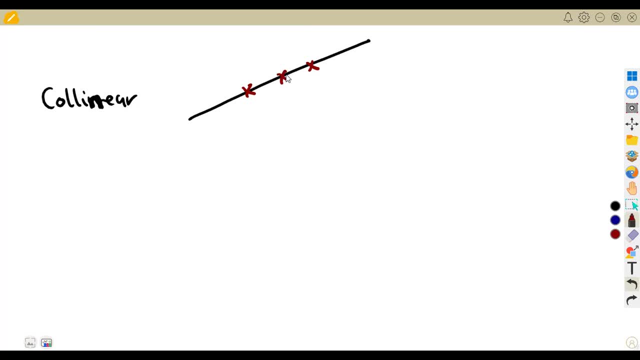 points. these points are on a straight line and they are co-linear. what it means is that from the first point, second point, the third point, i'm going to have the same gradient if i use any of the combinations. i can use the combination of the first point to the second point, okay. 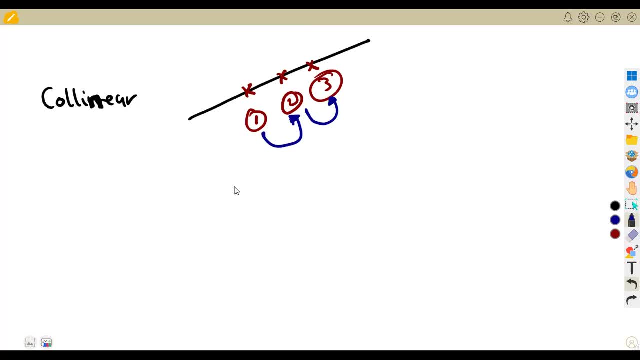 the combination of the second point to the third point, the combination of the first point to the third point. i'm going to have the same gradient. so the gradient that you're going to have between the points one and two, two and three- okay, one and three are the same. 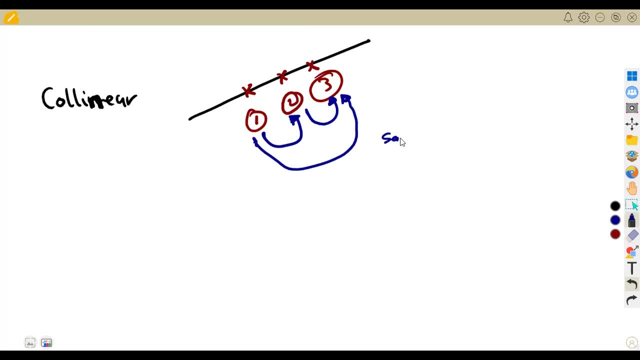 so that is for core linear. we are having what same gradient, same gradient, uh, throughout, throughout, the given point. all right, uh, the same gradient, uh, same gradient on the given, on the given, uh, on any given combination- let's just put that way- on any given combination. so, 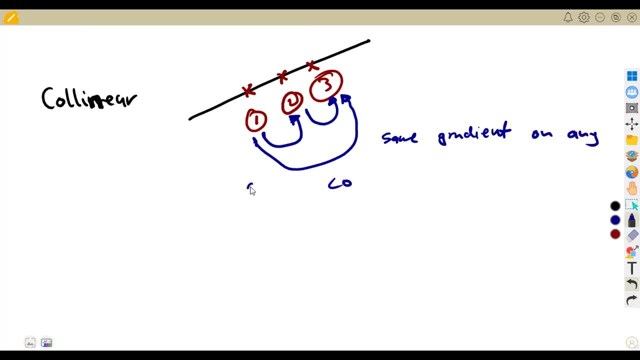 that you understand me properly. on any given combination, on any given combination, all right, that's it. on any given combination of a straight line, all right, that's it. on any given combination of a straight line. so, considering that i've got a straight line and there are points which lie on the straight line, 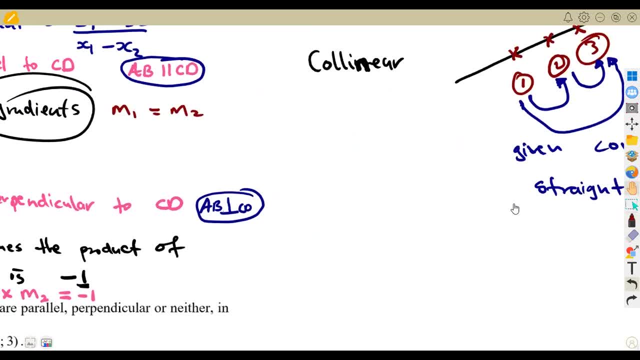 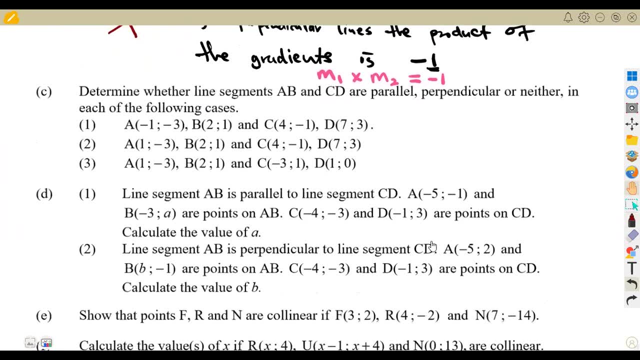 i'm going to use those points to determine just the gradient and equate that right. you see that you're going to have the same gradient, uh, throughout. okay, you're going to have the same gradient throughout. so these are the questions that you can have. uh, so you just want to check. 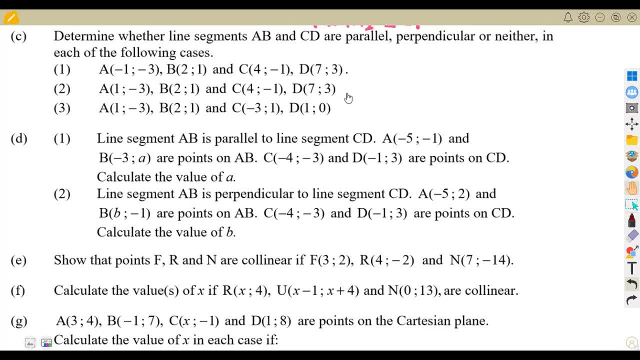 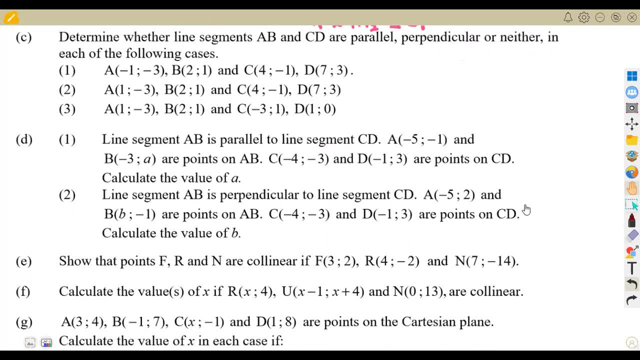 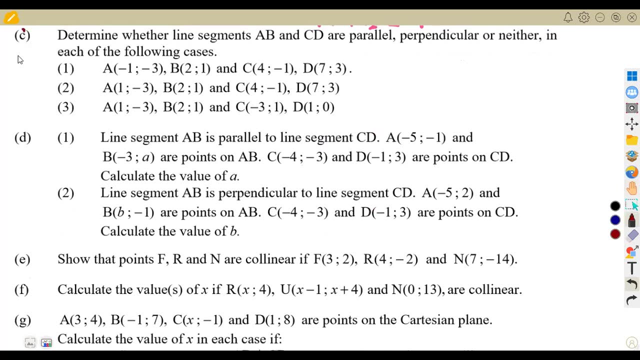 between what we talked about, the issue of the gradients and auciones. so you said these were also the uh- perpendicular lines, parallel lines and so forth and so forth. all right, so the first part of the question, which is uh c- all right, so this is the part c that we have of our questions- determine whether line segments a, b and cd. 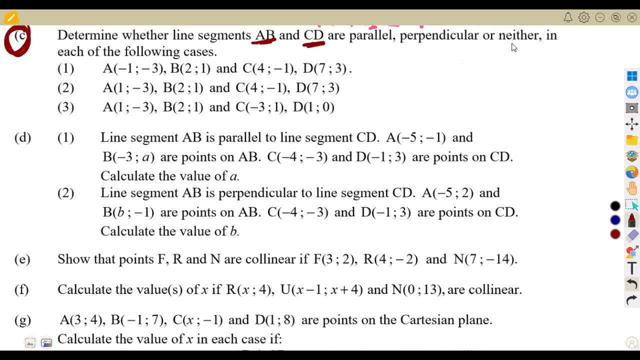 are parallel, all right. so this is the c one, to determine whether a, b and cd are parallel, perpendicular or neither. neither means not one of these. it's not parallel, parallel or it's not perpendicular. so that's it. so the c part that we have all right. so this is. 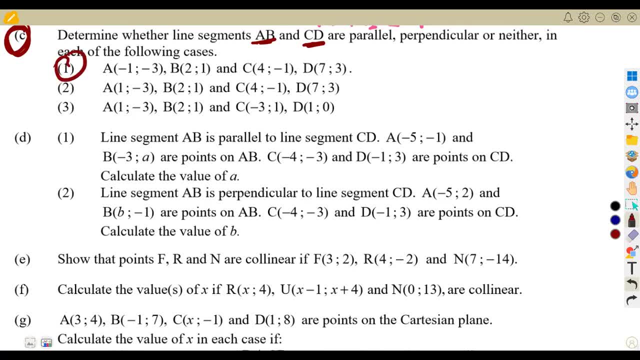 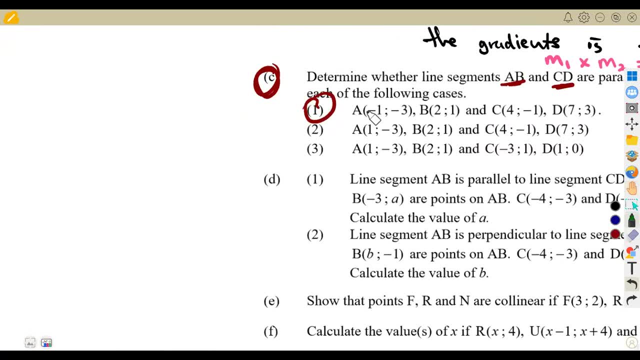 going to be c1, this one. i'm going to check this c1. uh, we've got two points, so this is how you take these points. there are two points that are given here. on number one: a b. remember we are comparing a, b and c- d. so this is our a b. the point a given as negative one. uh, negative three. this is our. 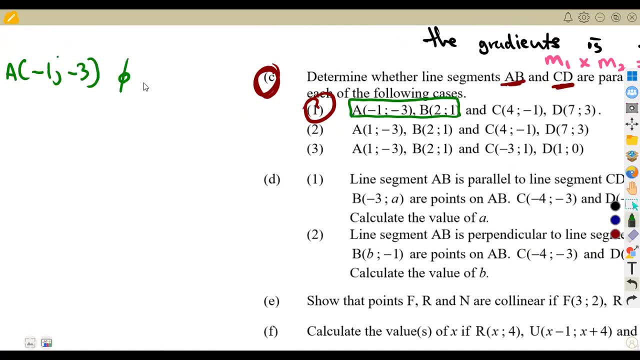 point a and i'm just gonna write in short, guys, okay, okay, let me just write end and end like this: and the point b, uh, the point c, d, in this case, this one from c to d, this second point that you have to compare with the point. oh, guys, i'm leaving the point b here, all right. two, one, i'm leaving the. 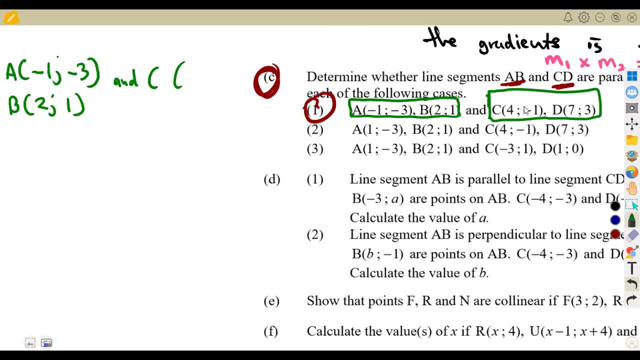 point by- i do not know what happened just there- c, which is four negative one, that's four negative one, and the point in d, which is seven three. so this is how you take your points. so there are two points here giving us a line, line a, b. there are two points giving us a line, line cd. it's a line cd, okay, line cd, line a. 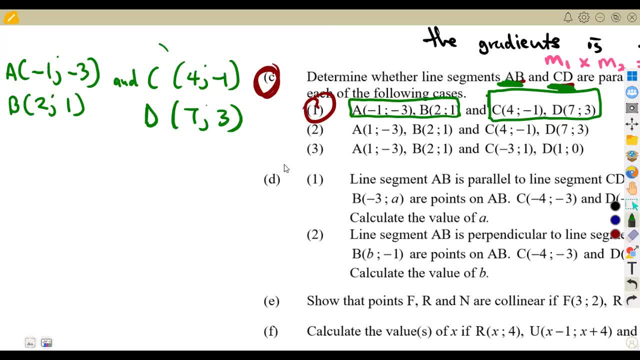 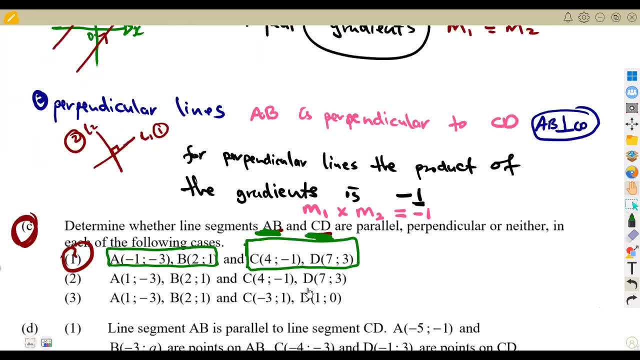 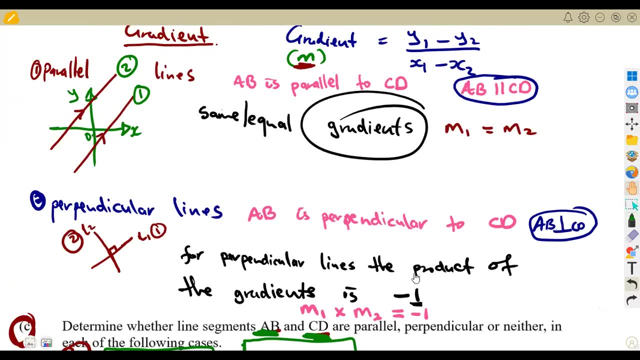 b. so it is given like: this is a line, line a, b, line cd. so we want to check if these lines are parallel, perpendicular or neither. so we said, for being parallel, what is it the condition? they must have the same gradients. they are perpendicular. the product of the gradients should be negative one. so if we multiply, 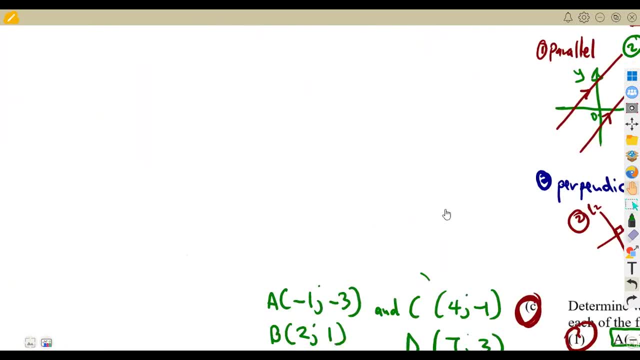 the product of the gradients. you must get a negative one if they are perpendicular. if they are parallel, we must have the same gradient, all right. so let's, let's do that and see what's going to happen. let's just want to put it somewhere here. all right, let's just put it somewhere here. 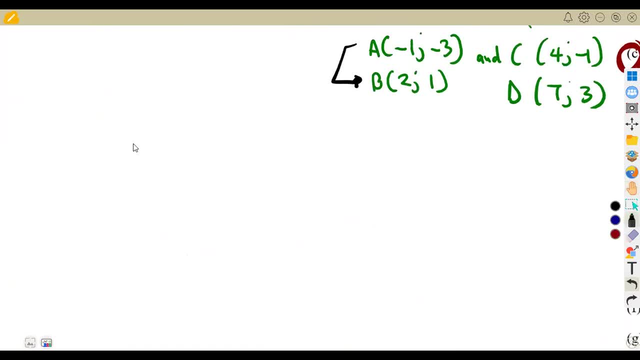 okay, this is what we have. we've got the point a and b. so remember i told you that the gradient you can just write in short as m, so you're going to have m a, b. the gradient of a- b, which we say the gradient of a line, is given by the change in y over the changing x, so that's y1 minus y2 over x1. 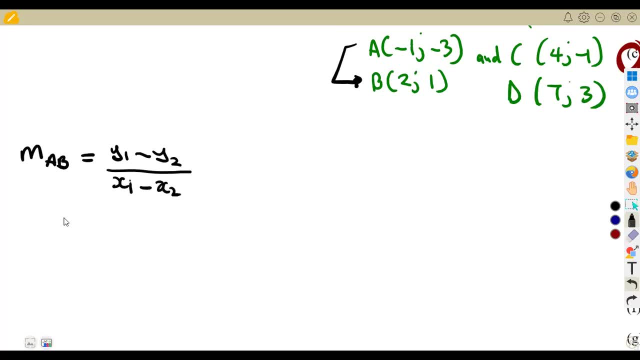 minus x2. so this is what you're going to have. what does it mean? it simply means on a, b, the point a and b. this is our first point. this is our second point. so i can just write this as my x one, this is my y1, this as my x 2 and this as my y2. so i've got x1 and y2. so here they arekum laser하다 x one. is our first point, this is our second point, so i can just write this as my x 1 and this as my y2. so, as my y1 is as my x 2 and this as my y2, so i've got x one. and why? if x has the same thing, uh, y is represented. 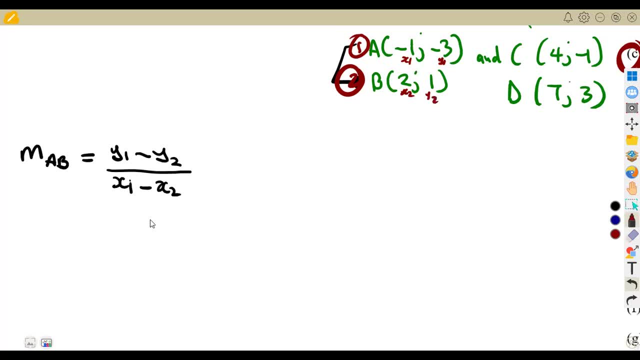 right x, truth be at the opposite of x, what you think. now i see why that large portion of x1 is��works. one on all of the and what, and x2. so this becomes my y2, x2, y2, x1, y1. that's the idea of the, the naming of the point. 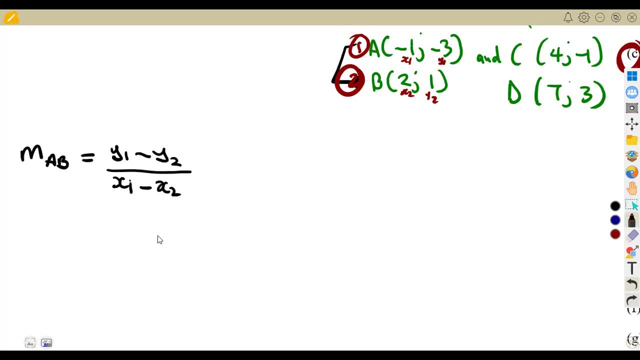 but as long you know, this is my first point, this, my second point, is not a metal effect. you can just substitute whatever that you have. so m i mean y1, which is a negative three. the y value from the first point is a negative three, minus the y value from the second point, which is a one. so that's one. 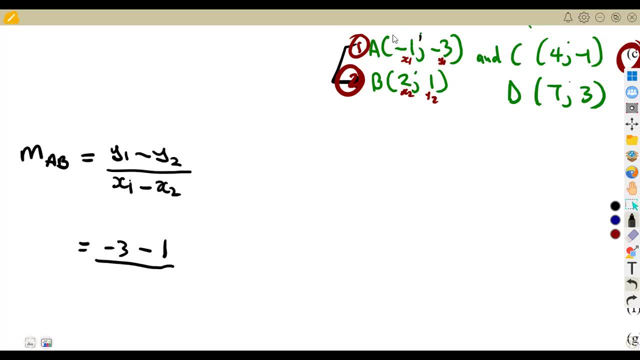 there over x1, the x value from the first point, that's a negative one. so you can just write negative one minus on our formula: the x value from the second point, which is x2. so x2 that is a two. so if you subtract this we are going to obtain, uh, the gradient of the straight line that we 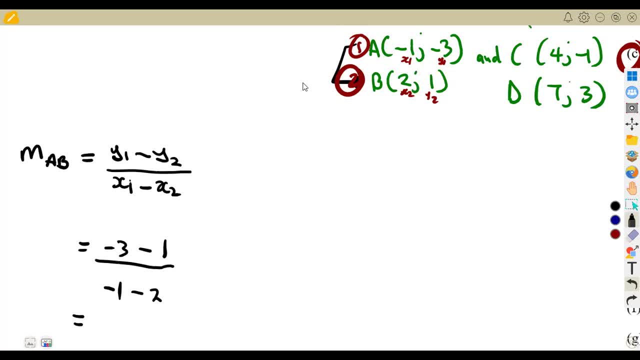 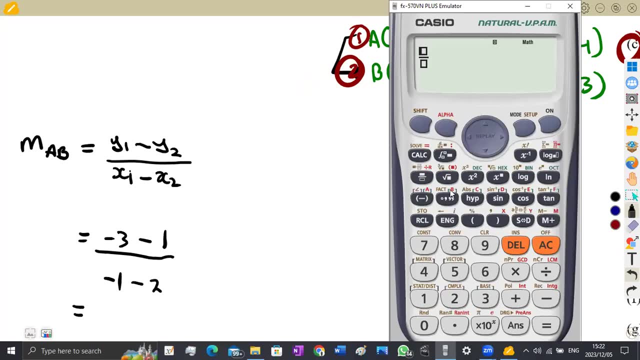 are given the gradient of what a, b, so let's just use the calculator, the calculator guys, at once. uh, no one is just gonna actually identify that you've used the calculator there, so just use the calculator straight forward. negative three, uh, negative one. negative three minus one, over minus one minus two. so this is negative one minus a two, like this. so this is. 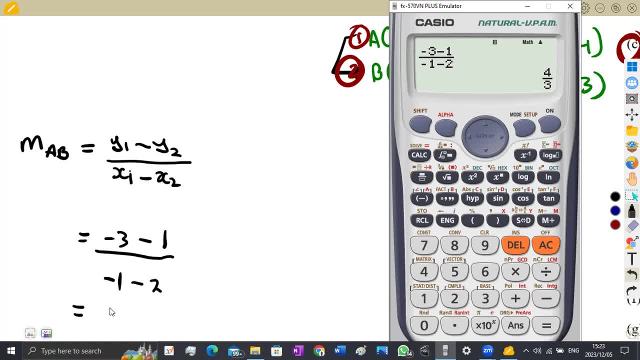 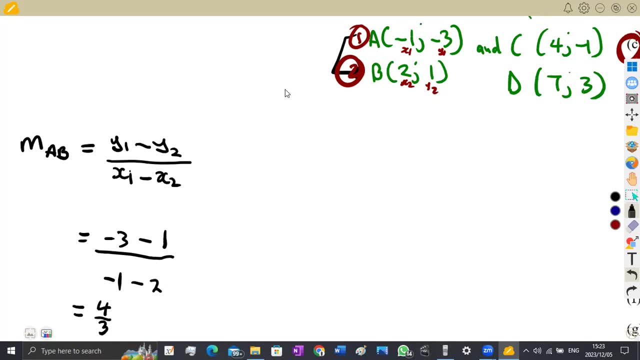 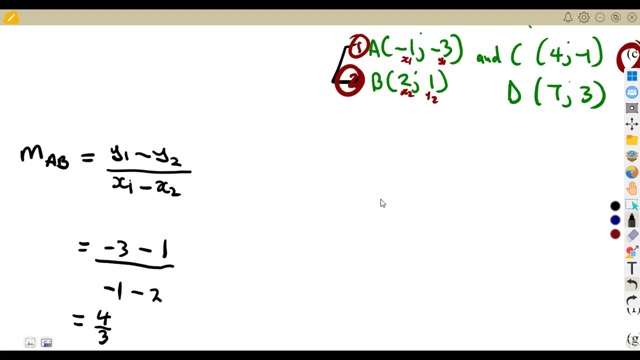 going to give us four over three, which is a positive. okay, so that's positive. uh, four over three. okay, just leave it like that. just leave it like that. remember, you are supposed to show, oh, you're supposed to to give a comparison. you are supposed to compare. 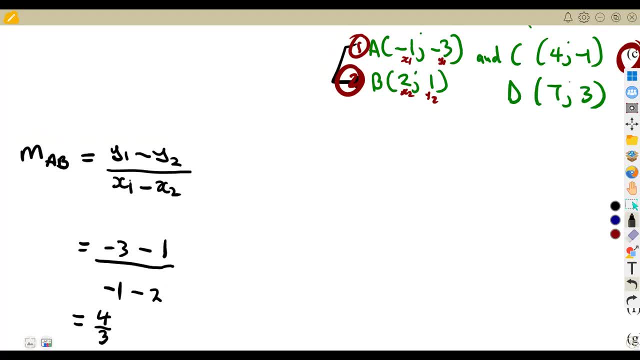 so just leave it like that. go to the other point, do the same thing. all right, let's go to the other point. we are now talking about cd. this is what we have, so we're going to calculate the gradient of cd, all right, so i've got the small letter m for. 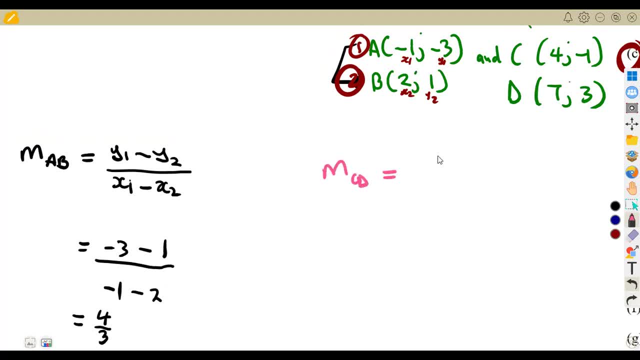 the gradient. this is cd. uh, that's gonna be again from our formula y1 minus y2 over x1 minus x2. we talked about this. let us just substitute, all right, so the same thing. this is your first point. your second point. so as long you know that this is the x, this is the y, you can write: yes. 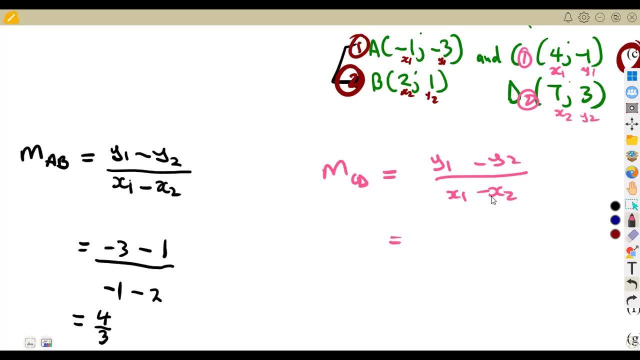 this one. let's just write so that all of us we follow suit. okay, so that's y1, which is negative one. so that's negative one minus y2, y2, which is a three, all right over x1, our x1 there, which is a 4. 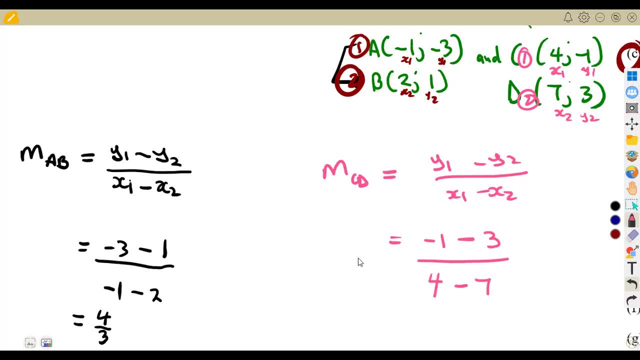 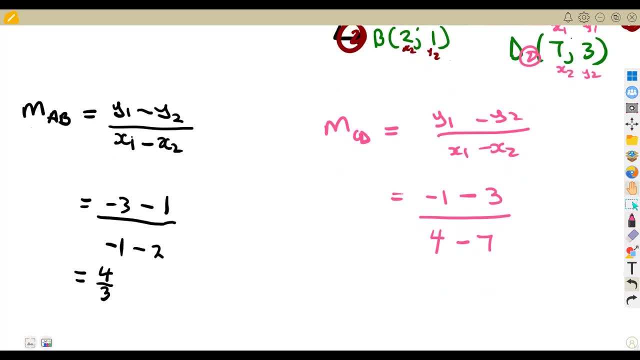 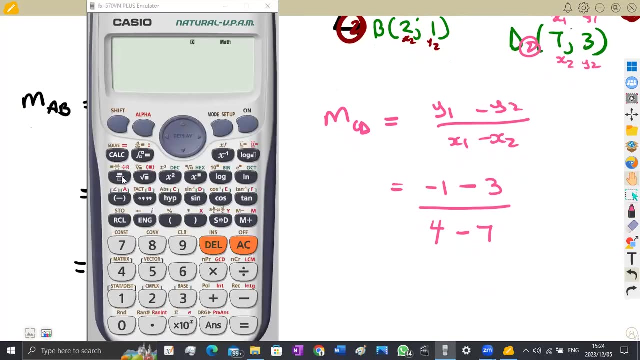 minus x2, our x2 here, which is what? which is a seven. so let us subtract and see what we are going to have. in fact, let's just simplify everything straightforward on our calculator so this can help us to be fast also. all right, so this is what we have just put: a fraction. 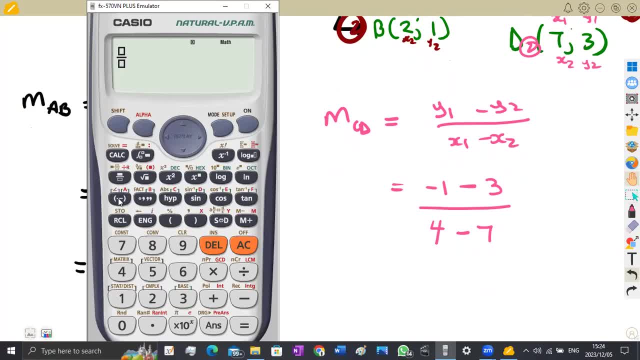 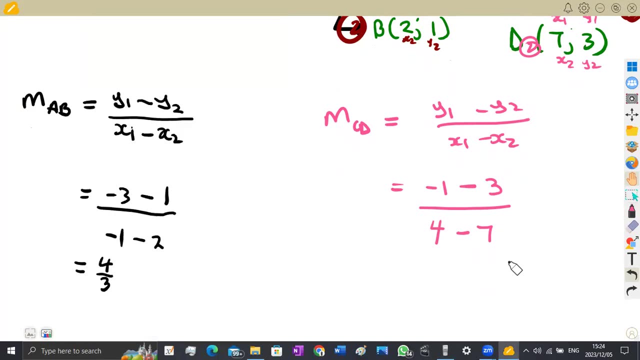 and that's negative. one minus three- okay, so that's a negative here. one minus a three. four minus seven. okay, in the denominator we're gonna have four minus a seven and this gives us a four over three. okay, so this is what we're going to have here. okay, this is what we're. 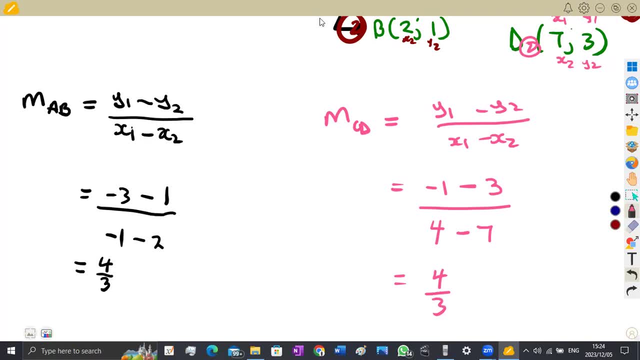 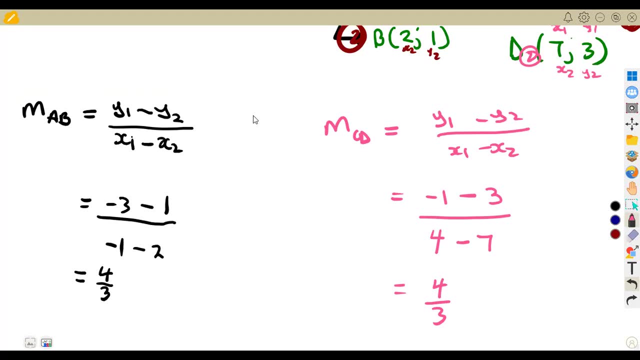 going to give us a four over three. now that we have got two gradients, we can compare them. remember the idea there is on was on the comparison. you want to check whether they are parallel, perpendicular or not. remember what i say on terms of the gradients. if the gradient 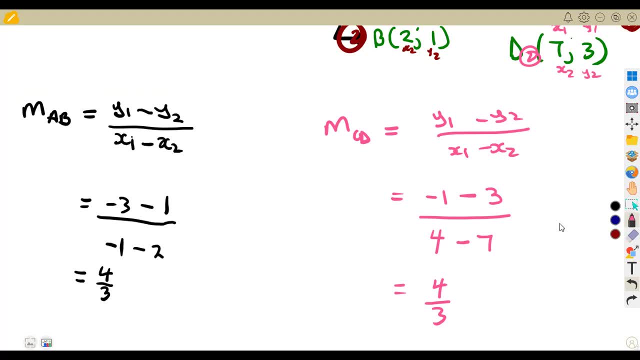 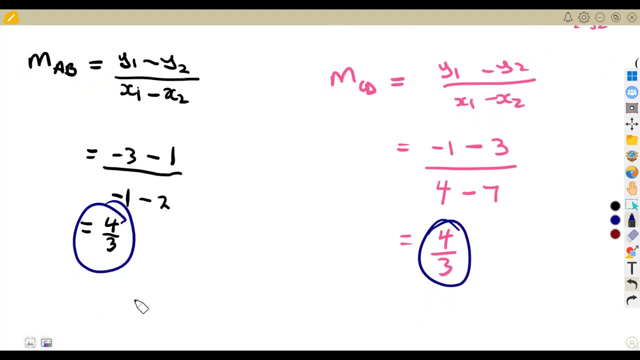 are the same. what does it mean? it means these two lines. they are parallel to each other. we've got four over three and four over three. they are the same. so therefore, from the first condition that we have a, b, uh, a b. all right, let us just say, since, first, since, uh, the gradient of a, b is equal. 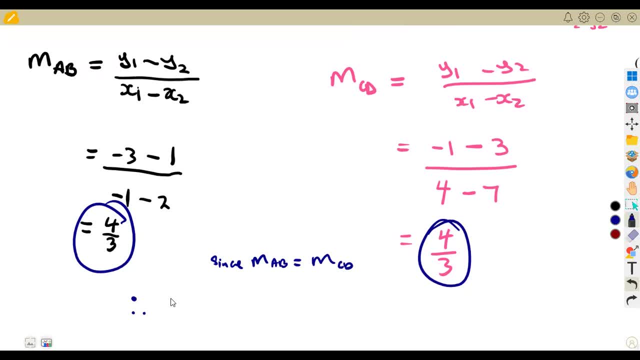 to the gradient of c d. therefore the line a b is parallel to add to c d. remember we said we can write the parallel sign in short, like that. so we are simply saying these two lines, they are parallel to each other, why they have same gradient, same gradient. 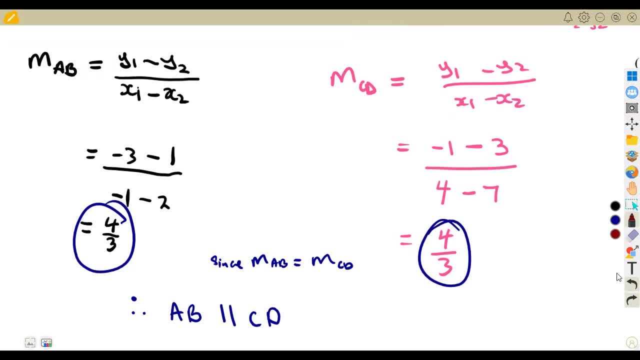 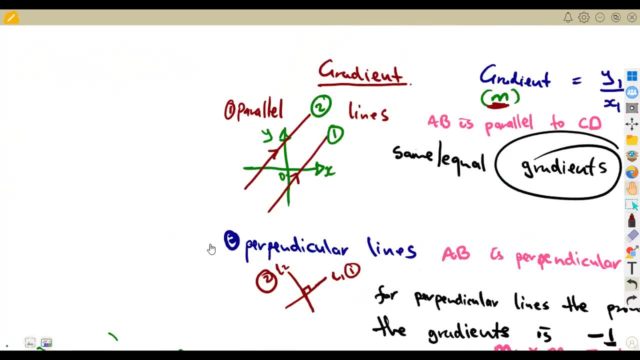 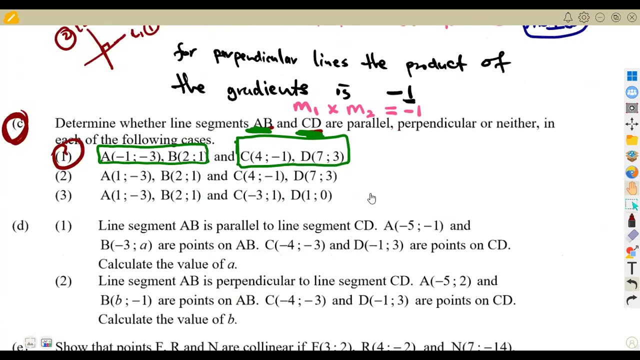 same gradient, parallel, okay, what if they were perpendicular? the product of the gradient should give us a negative one, like i said here. for what? for perpendicular lines, the product of the gradient should give us a negative one. so try. i want you to try. what is going to happen? 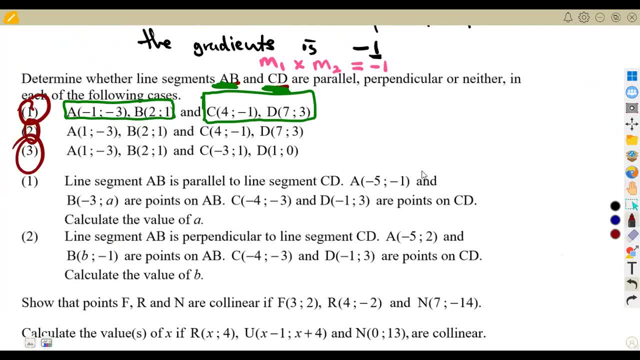 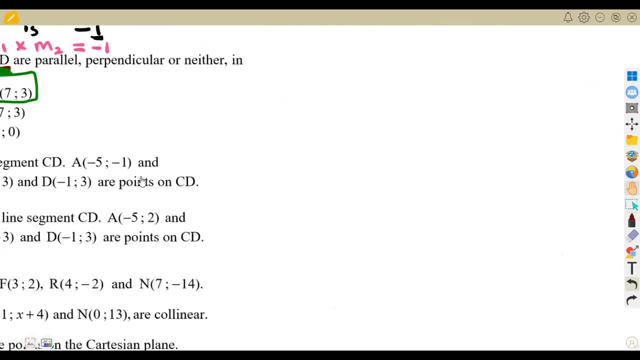 with, uh, number two, i'm just gonna try number three with you, all right, so you're gonna have the same thing, or number three for the point a, which is one minus three. all right, the point a. let me just write our points aside. the point a, that is one minus three. so, like i said, i'm just gonna try number three. 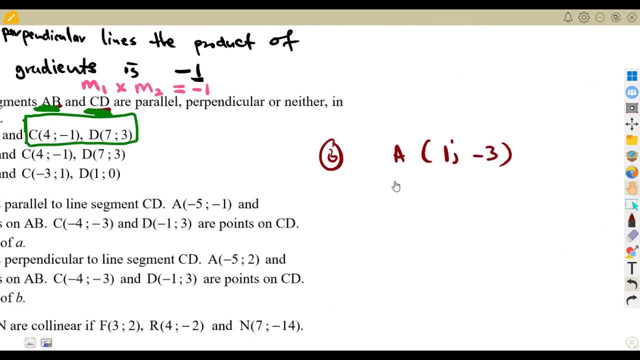 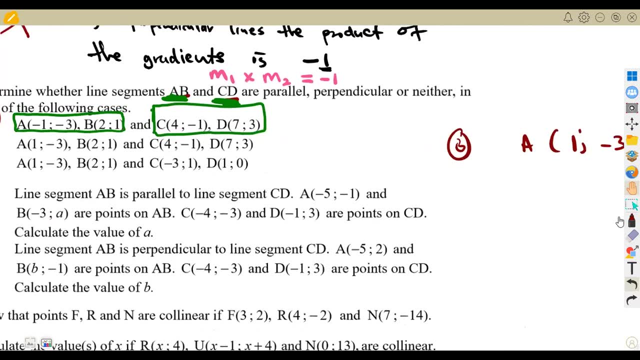 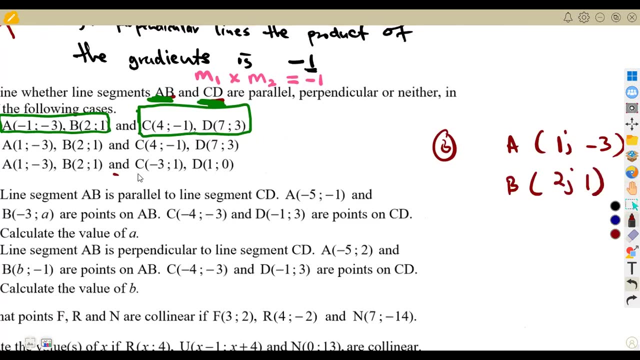 with you guys. you try number two, all right, and the point b there. on number three, the point b, uh, is two one. the point b is two one. let me just write it aside here. point b is given as two one. okay, then cd on this part. the point c is negative: three one. 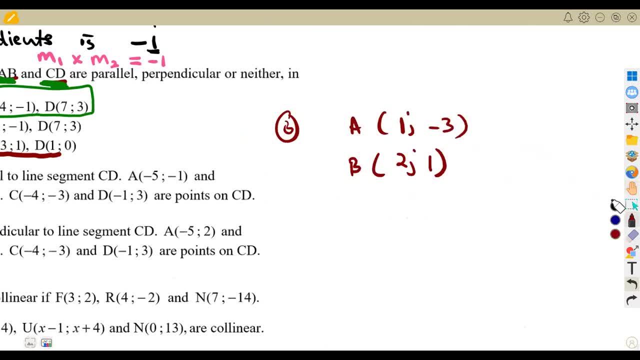 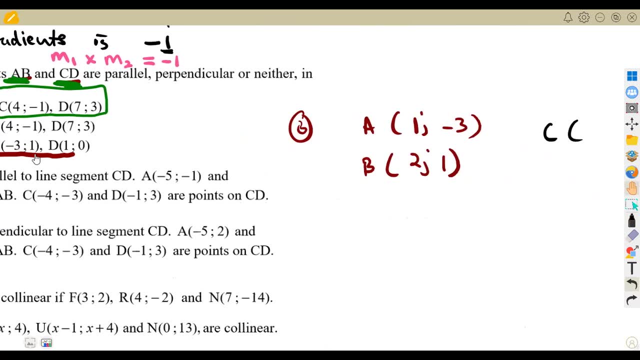 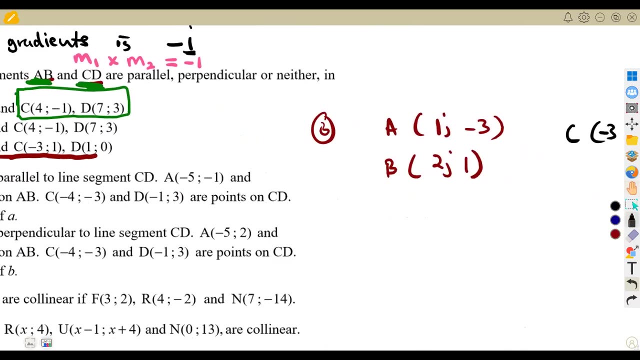 okay, the point c there. on the other hand, you've got a point c, which is three, one. is it three or negative three? that's a negative three. you see, i'm hiding this one, i'm hiding it, but the negative three there. so we've got a negative three versus one. okay, negative three versus one. 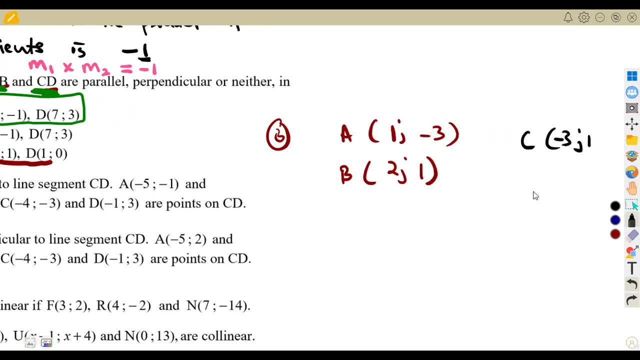 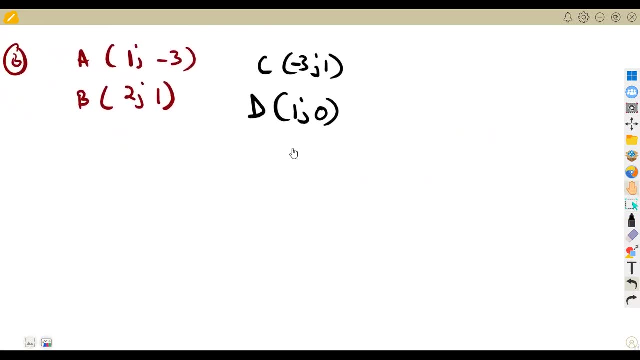 oh, like this. then also the point d given the point d, one zero. the point d given as what is one zero like that. so this is what we have, all right, that's number three. you want to check if these two lines are parallel or not parallel, perpendicular or 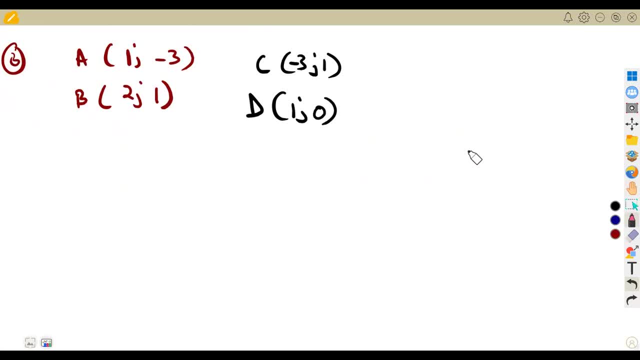 neither of those. okay, cannot be perpendicular, it cannot be parallel, it can just be a normal line, not perpendicular, because if these two lines, those two lines can meet, but they can meet maybe at 60 degrees, not at 90, because to meet at 90 degrees, that is to say they are what happened, parallel, they're like 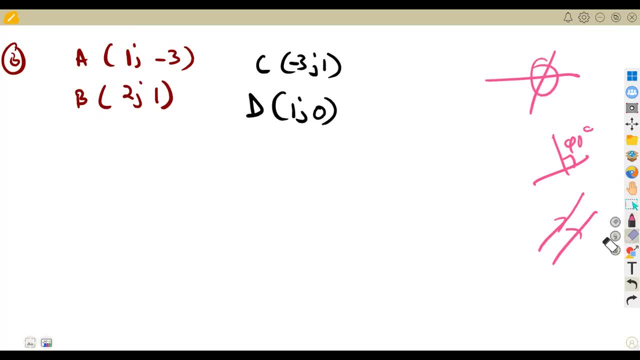 this, they never meet. but if they meet like this, we do not have a special uh consideration that we can use uh to tell in terms of the gradient. the only thing that we can use to tell if the two lines do intersect uh is on a condition whereby you are solving the, the equations of the given line simultaneously. 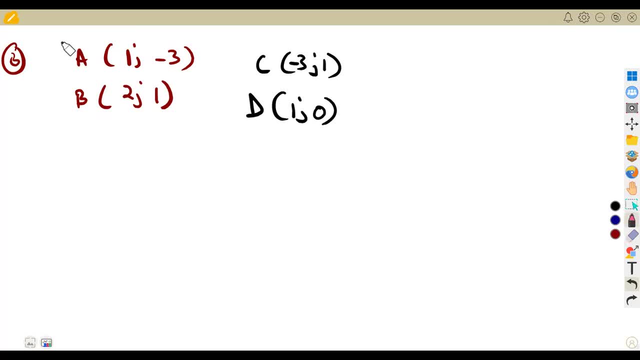 the same that we want. on functions, we talked about that, but here it's another. that's another thing else, all right, we talk about the gradients. so let's calculate our gradient and see if what a, b, just like the previous case. remember, we said we can just write this current of. 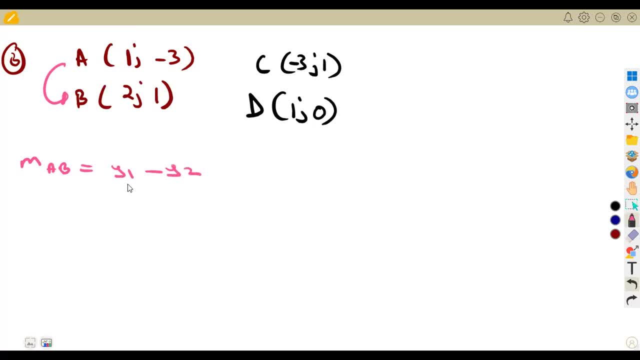 a, b from the formula y 1 minus y 2 over x 1 minus x 2. it means, uh, this a can be my first point, all right, b can be my second point. so i've got x 1 or y 1 here. i've got x 2 and i've got y 2, so y 1 being a negative 3. so i'm going to have 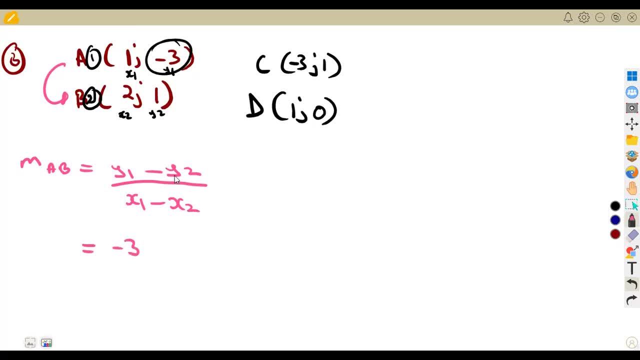 this as negative: 3 for y 1 minus y 2, so that's minus y 2. the y value, uh, at the second point is 1, so that's minus 3, uh, minus 1. okay, over x 1. so you're going to move to x 1, the x value from the first point, which is a. 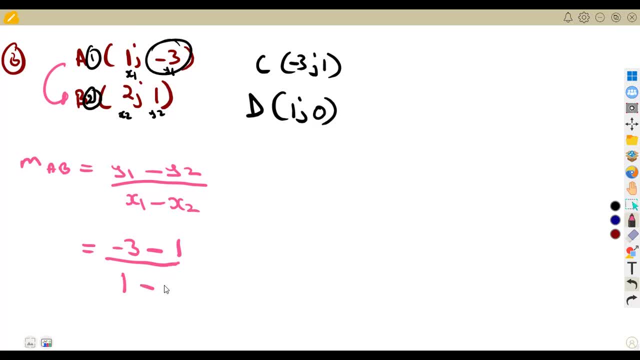 1 minus x 2, the x value from the second point, which is a 2. so let's subtract and see: minus 3 minus 1 over 1 minus 2, that's going to be minus 4 over minus 1, which is a 4 right. so this gives. 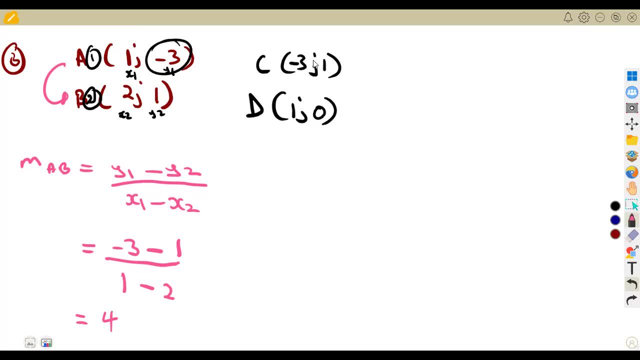 us a 4, or we can just use our calculator because, uh, to avoid, just just to avoid, mistakes, all right, because sometimes you know you're in exam, this and that thing happen, uh, in exam. you know, a lot of things can just happen during the time of. 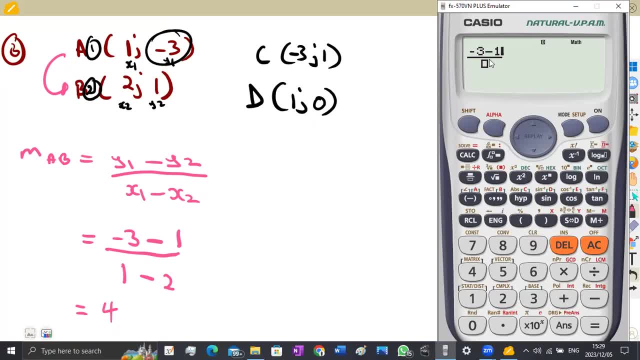 exams or even in it on a normal day. all right, so minus 3 minus 1 over 1 minus 2, this is going to give us what? uh, that's minus 2. okay, so this gives us a 4. okay, so, like just the previous class, let's. 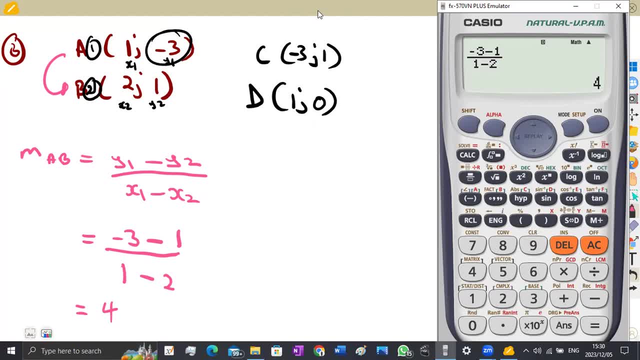 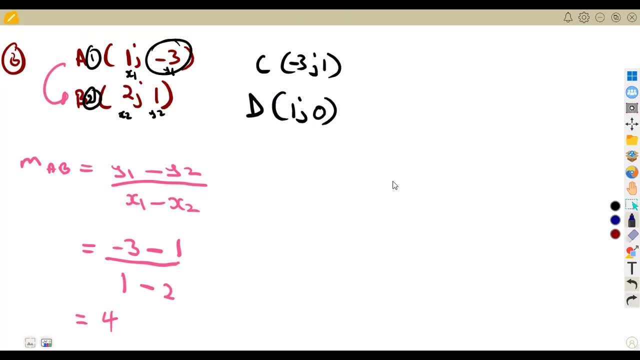 say, this is just going to be a positive form. so, as you can see, just use the calculator for the proof, or you can just simplify it direct from the calculator, which is fine. so it moves on to the second point, which is our cd, i mean the second line. so you're going to have the gradient. 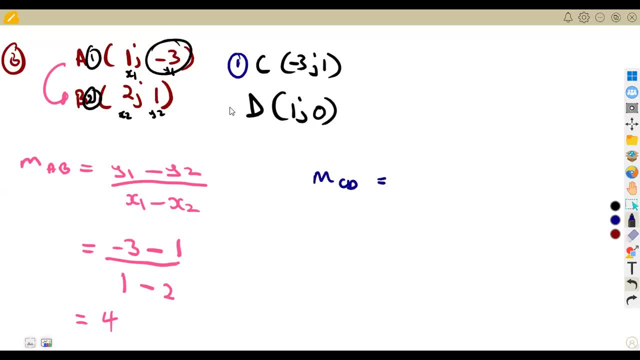 of cd in that case. so let us consider, say this is our first point or second point. so you're going to have x 1, y 1, x 2, y 2 from the second point, so from the gradient y 1 minus y 2, so y 1, here is a 1. 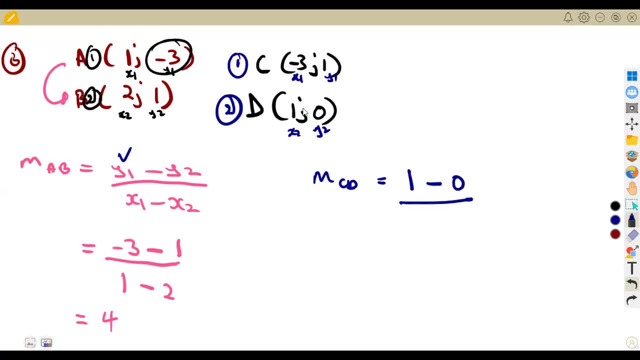 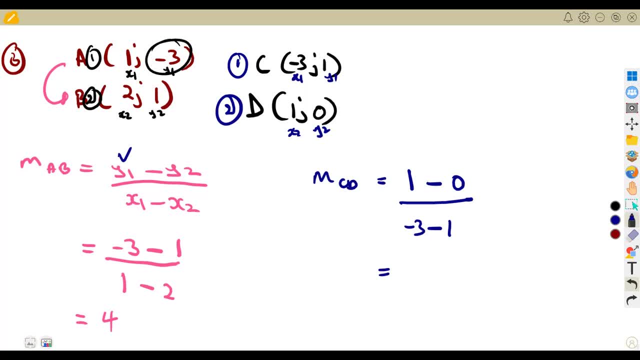 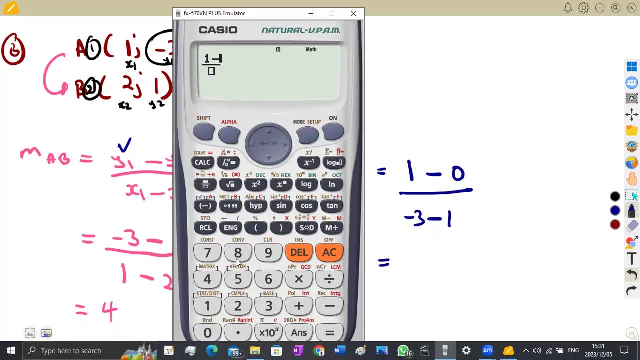 uh, cd in that case? okay. so let's determine the gradient of the line cd on our calculator. just going to have a fraction: 1 minus 0, which is a 1- okay, over minus 3 minus 1, which is minus 4, okay, anyways. let's see minus 3 minus 1, like this. this is going to give us negative 1. 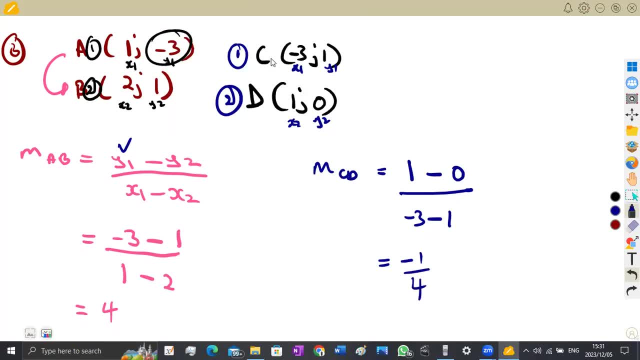 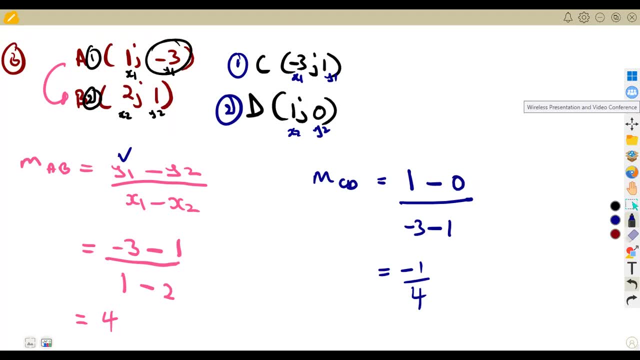 4 negative, 1 over 4, like that. so the question is: are these lines parallel? because now we have got the gradients. so you have to ask yourself now: are these two lines parallel? no, no, they are not. they are not why why? because the gradients are not the same. we only stock of parallel lines if the 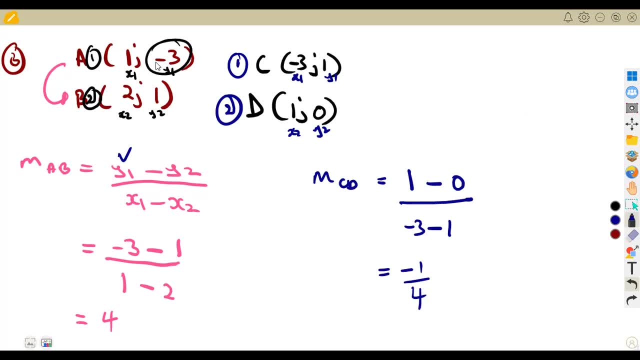 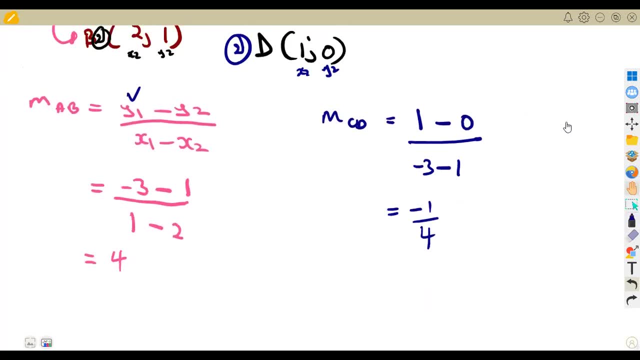 gradients are the same. so here the gradients are not the same, so they are not parallel. so what are they? we move on to the second thing. it's either we are talking about parallel or being perpendicular. so when being perpendicular? now we prove with the product of the gradients. 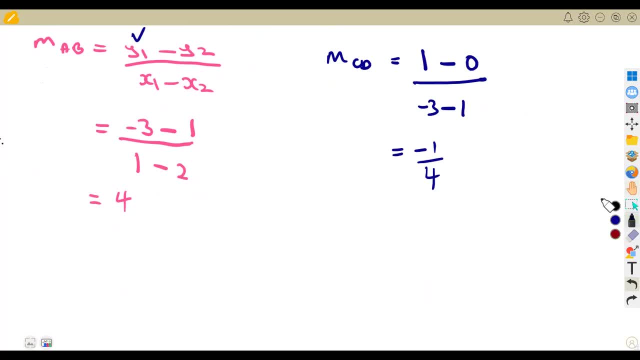 what are we going to get if we get a negative one? therefore they are perpendicular, but let's check. so we're going to check the gradient of a, d, of a- b times the gradient of cd that we calculated. the gradient of a- b gave us a four right, so that's a four times the gradient of cd here, which gave 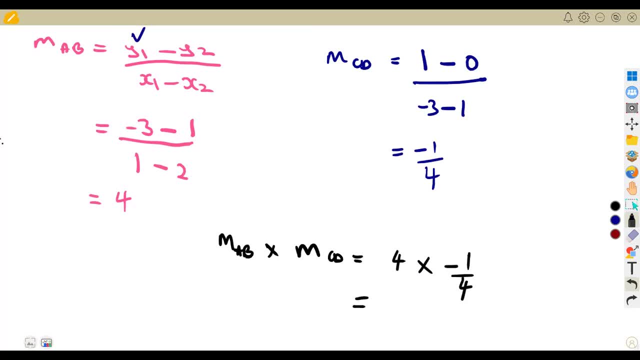 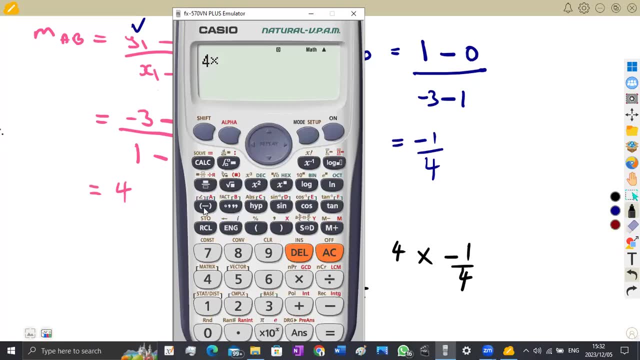 us negative one over four. so if you multiply properly on our calculator, this gives us a negative one. yes, let's just do it. cycle free vision on our calculator. so that's four times a negative one over four times negative one over four like this. negative one over four like this: this gives us negative one. so we are going to obtain a negative. 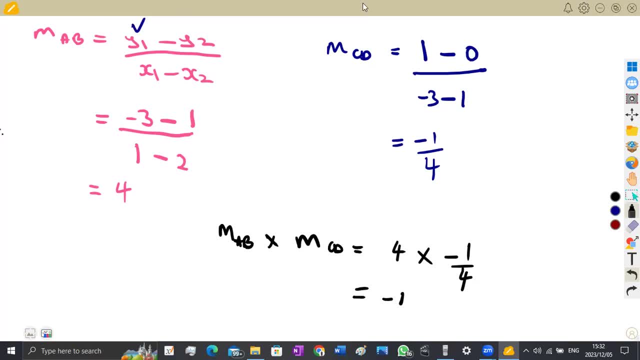 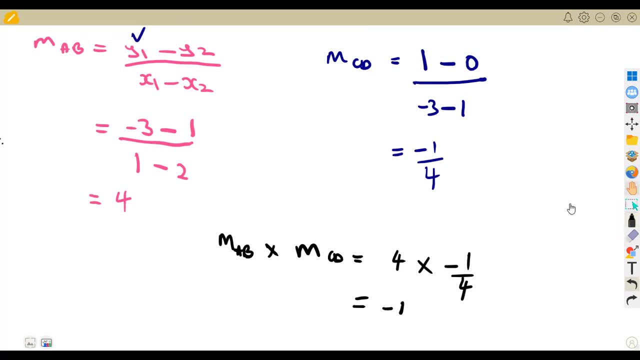 one, so obtaining negative one. what does it mean? that is the question. what does it mean to obtain a negative? it means these two lines, they are perpendicular, remember we say perpendicular lines. the product of their gradients is what is a negative one. if you multiply their gradients, you are going to get what a negative one. so by multiplying these two gradients, that 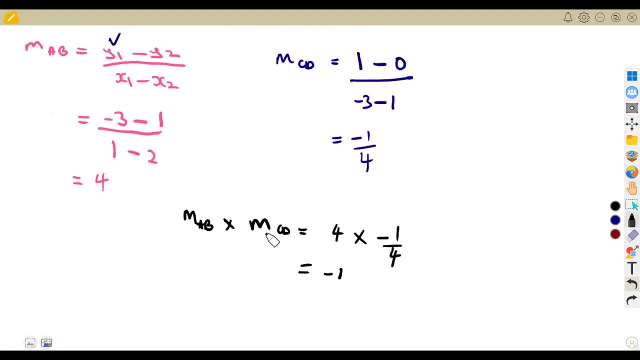 we have the gradient of line a, b and the gradient of line cd. we got a negative one, so therefore it means a- the line ab is perpendicular to the line cd. all right, remember this is the symbol for being perpendicular. so that's how you can check whether the two lines 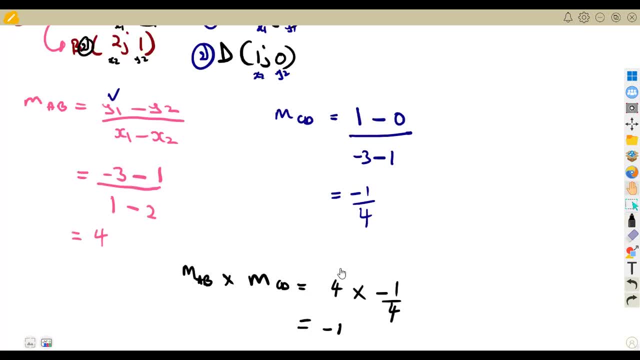 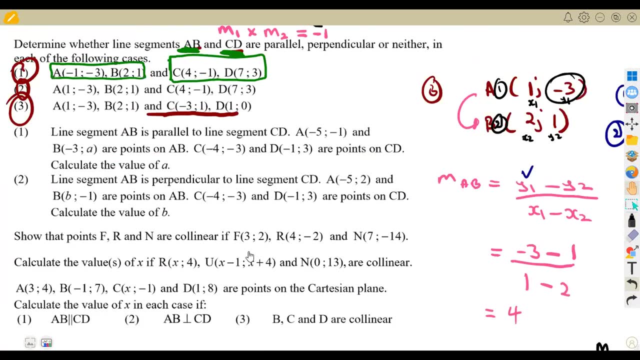 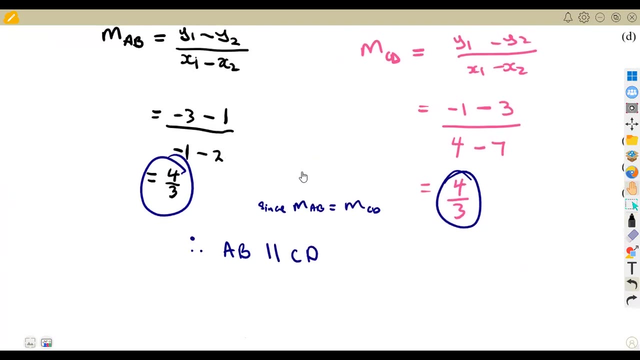 that you're dealing with are perpendicular or parallel. okay, so this is a condition when they are perpendicular- the previous one. we saw that if they are parallel, you consider the idea of what equal gradients, like we calculated here. we saw that these two lines they gave us equal, equal. 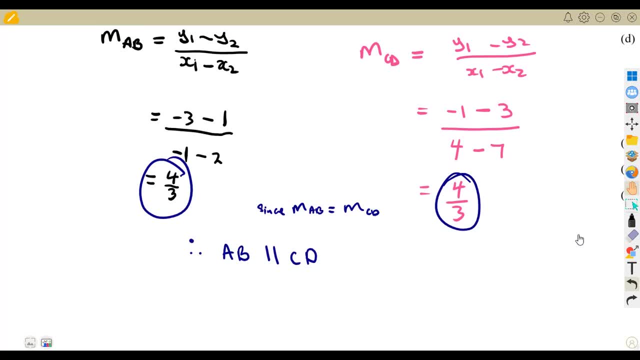 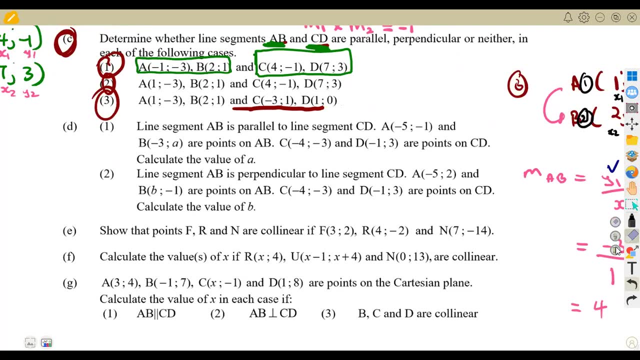 equal gradients. four over three. four over three, all right, so that's it. you're gonna check as much as you can so that you just work out to see how do they ask the questions. remember i also talked about being called linear uh, whereby we've got the same gradient throughout. 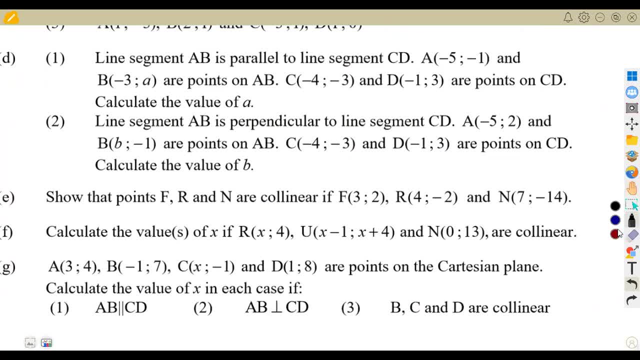 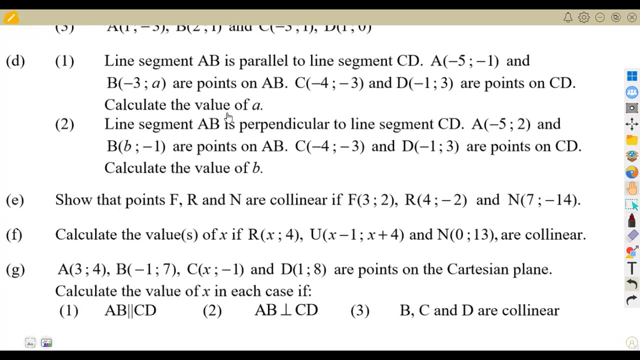 but let's check, uh, d it was. let's see this person. uh, it can be it, it can be of chance to be done. uh, line segment ab is parallel to line segment cd and okay, this one is a very, very important question. okay, let's see this person. they are saying the line segment this is d1. okay, so we're talking. 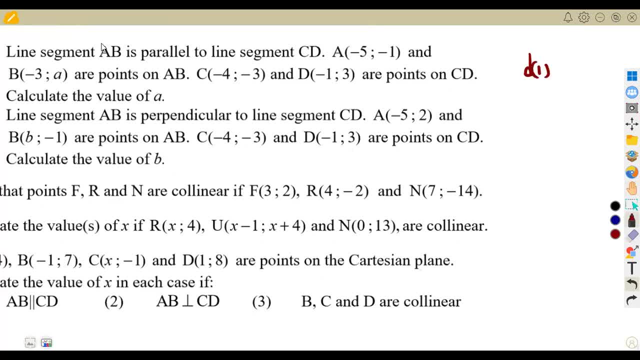 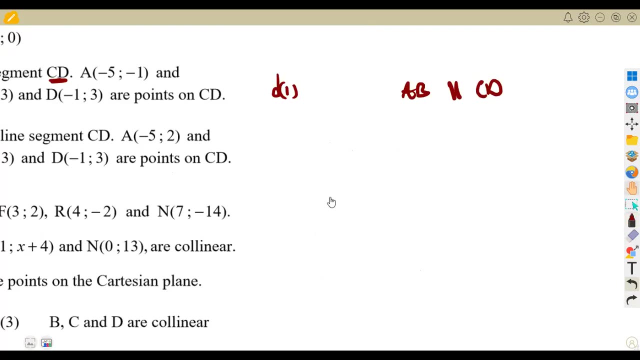 about person d1. they are saying the line segment a, b is parallel to the line segment cd. all right, so a, b is parallel to cd. this is what we are told. a, b is parallel to cd. remember we say this is the symbol for being parallel a we are given the point. 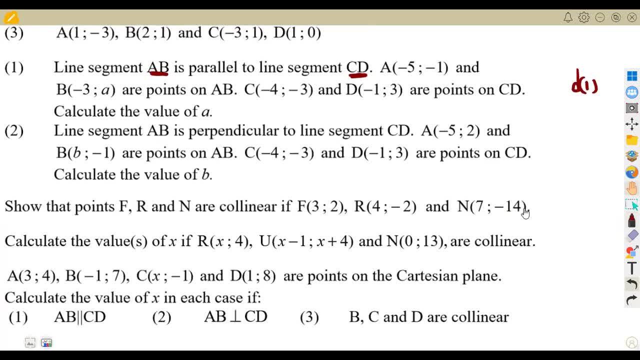 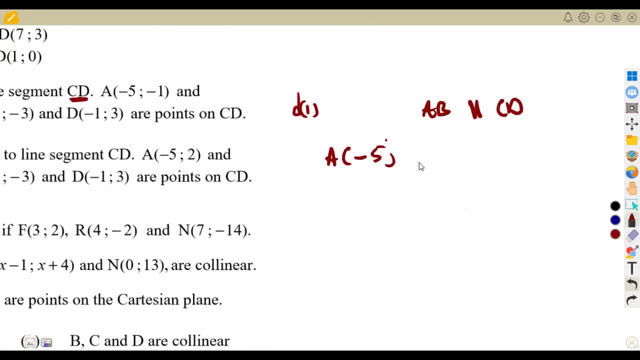 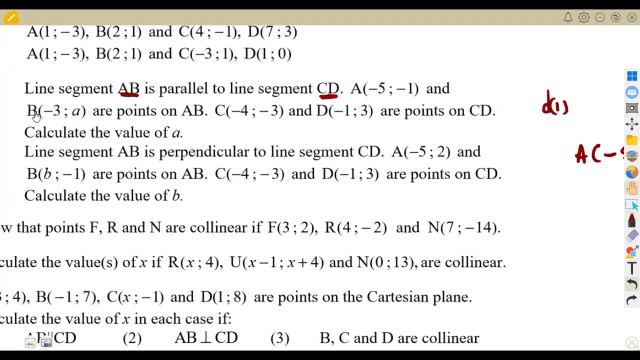 a and the point b, a minus five, minus one, all right. so the point a is given as negative five, negative one, and the Point B is given as there's an unknown value there to be negative 3A. So we're given negative 3A like that, all right. 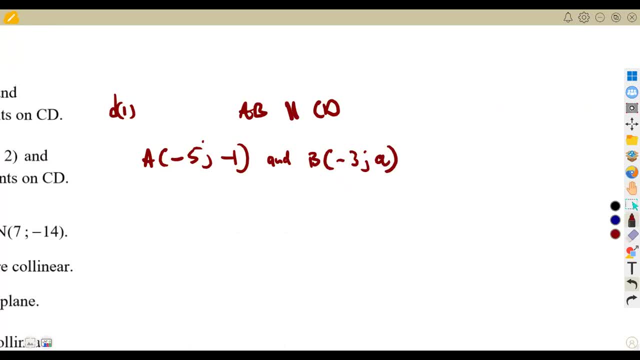 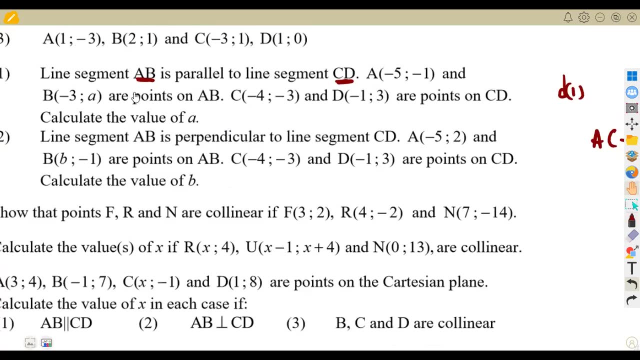 This is our point B, negative 3A. Okay, and we move on to the point C D, to the line C D. all right, These are the points that are on AB. okay, A and B are on AB. the line AB: all right. 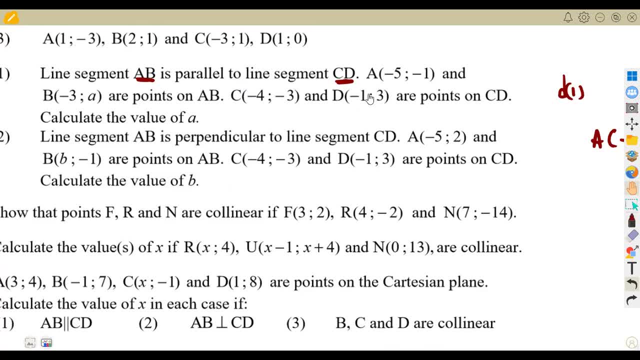 And we have got the point now. C and D, which are on CD, Calculate the value of what of A? calculate the value of A. Okay, let us take the points that we have on CD. We are told that on CD, the points that we have is what? 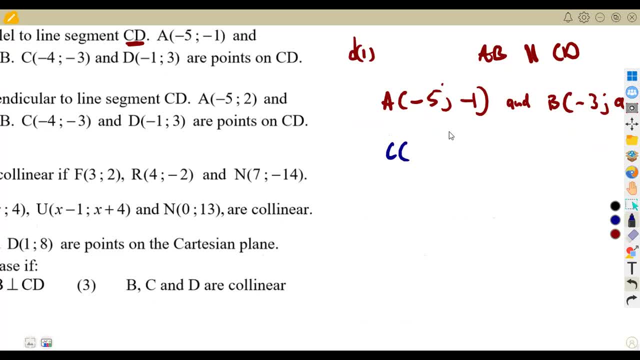 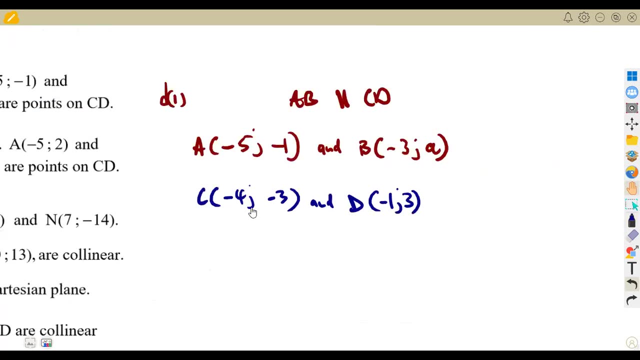 Is C negative 4, negative 3, and the point D being negative 1, 3.. This is what we have, and the question there was to calculate the value of A or to determine the value of A if these two are parallel. 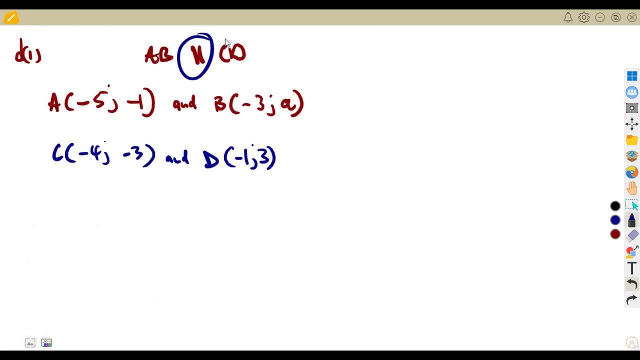 Remember, there's a condition given, So you work with the given condition. What is the condition? What is the condition? They are parallel lines. So what is it that I know about these parallel lines? There is something that we know. What is it? 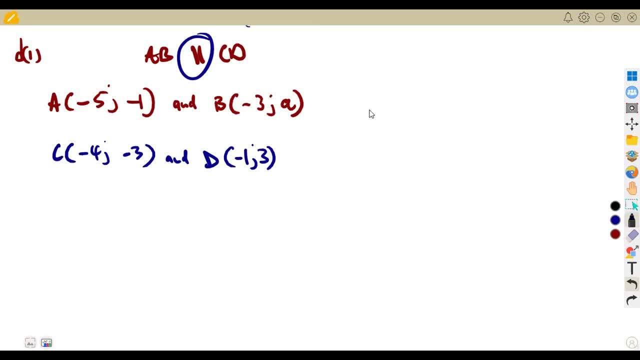 We use that To our advantage. now, What is it that we know? We know that they have got the same gradient. The gradient of AB must be equal to the gradient of what? Of CD. in short, Just going to use M for the gradient. 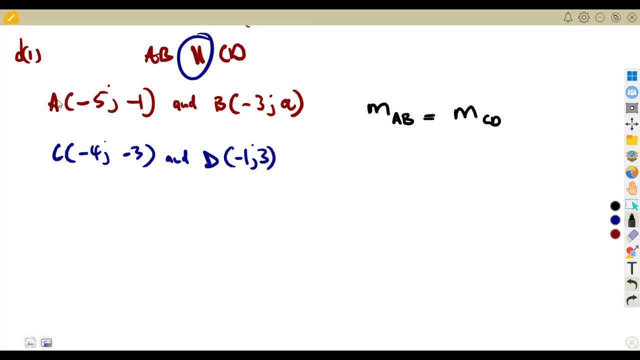 So it means, if I calculate the gradient of A and B, these two points here, A and B- Okay, let's calculate it, The gradient of AB. I'm going to calculate this in terms of A, because I'm supposed to calculate the value of A. 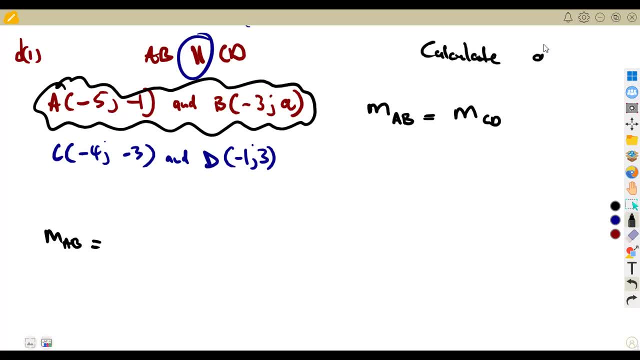 Remember- That's our question- Calculate the value of A. So gradient, as we know, we say the gradient is the change in Y over the change in X, That's Y2.. Y1 minus Y2 there over X1 minus X2.. 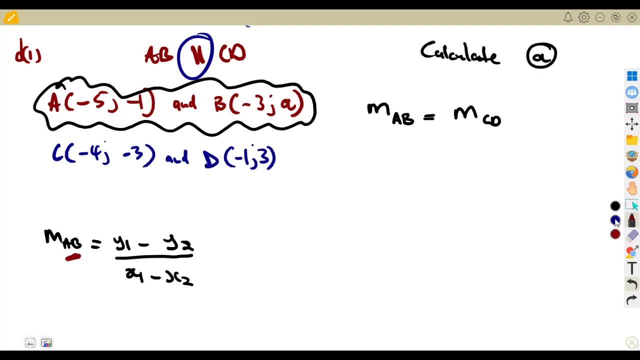 But we are considering AB, the line AB. So, on AB, this can be your X1.. This can be your Y1.. This can be your X2.. This can be your Y2.. So you can just substitute on your formula, since you wrote. 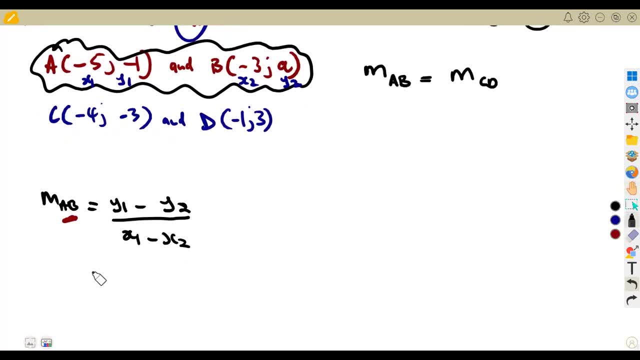 Y1 minus Y2.. Depending on the formula that you are using, you can use: Y2 minus Y1 is one and the same thing, So Y1 is negative 1.. So that's negative 1 minus Y2.. Y2 is given as A. 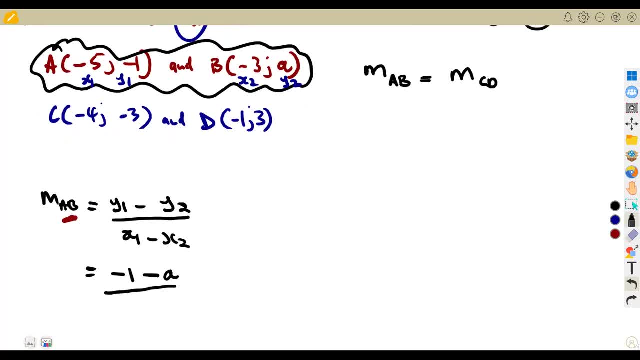 Everything over X1 minus X2.. So you're going to have, in this case, our X1, which is negative 5.. Remember, we are on AB, So the X on AB there is It's negative 5.. That's our X1.. 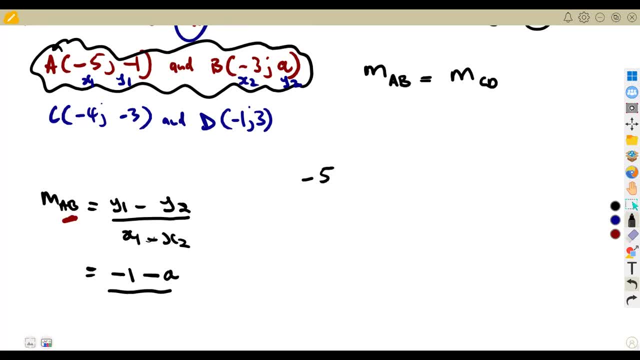 So it was supposed to be minus 5, minus X2.. All right, That's our formula: Minus X2.. What is the X2?? Our X2 is minus 3, guys, We have talked about this, So we're going to have minus 5 minus minus 3, which is a plus. 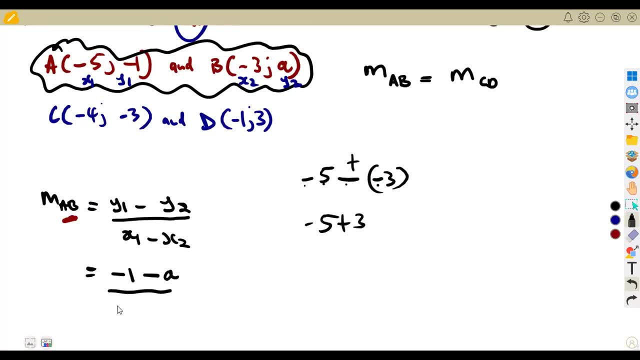 So we've got minus 5 plus 3 for this one. So this is going to be minus 5 plus 3, which is minus 5 plus 3.. That's a negative 2.. Yeah, something like that. That's a negative 2.. 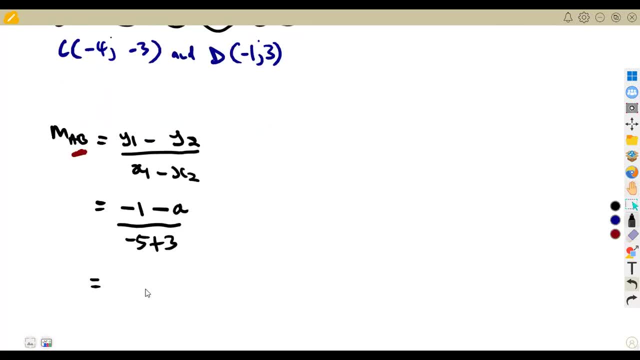 So you're going to have This as minus 1 minus A, Minus 1 minus A over. We said minus 5 plus 3. That's a minus 2. Check with your calculator also. So that's a negative 2.. 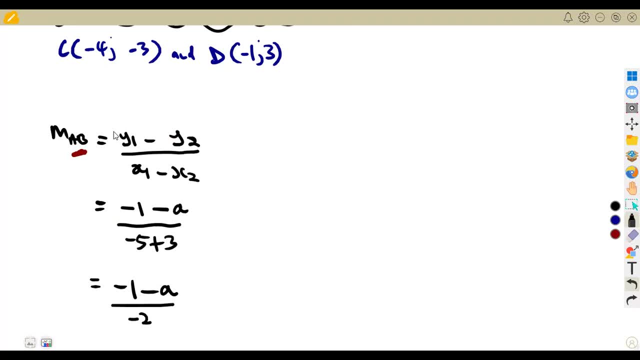 All right, We are together now. So now that we have the gradient of AB- remember we are told that these two lines are parallel- So I have to calculate also the gradient of CB so that I can be able to Use the gradient concept, because we talked about this. 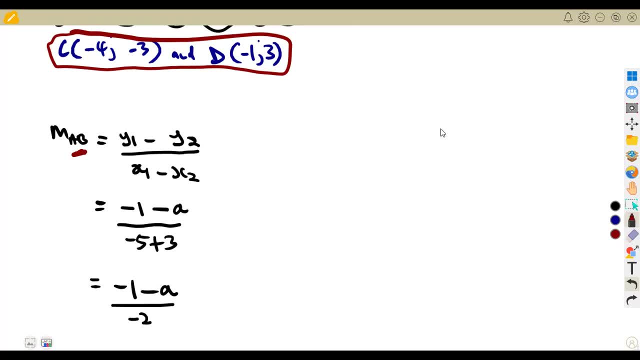 If two lines are parallel, the only thing that you're supposed to think of is the gradients. So let's calculate the gradient of CD. The gradient of CD, this one, is going to be what Same thing, Going to have our X1 from the first point, second point, X2, Y2.. 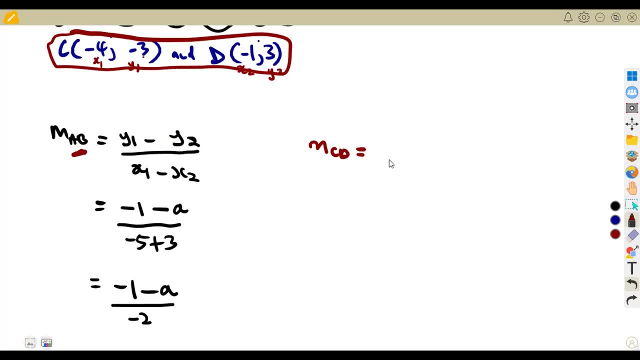 So that's going to be Y1 minus Y2.. So Y1, that's a minus 3. Minus Y2.. Y2, in this case, here is a 3. Over X1, the X1, the X value at the first point is minus 4.. 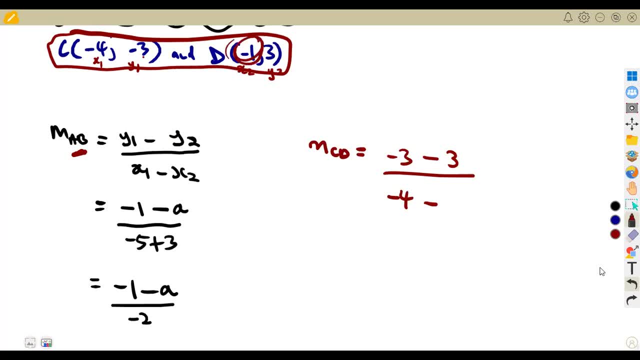 Minus X2, X2, in this case from the second point, is a minus 1.. All right, I wanted to avoid this thing of negative, negative like that. Okay, Anyways, that's minus 4 minus minus 1, which is a plus. 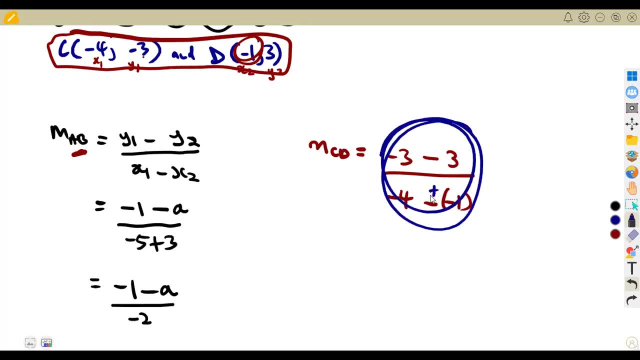 So this is just going to be a plus. And also take note, these are numerical, numerical values. It's not an algebraic, It's algebraic Expression where there is A. you can't simplify 1 minus A, Minus 1 minus A. 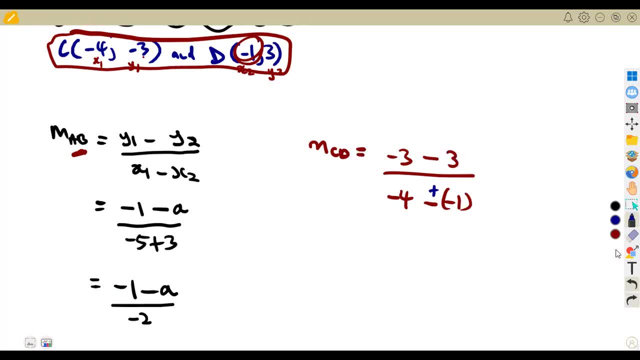 But you can simplify these numbers, numerical values. we are used to these numbers, So let's simplify them on the calculator and see what you're going to have at the end. So remember just going to have a fraction minus 3, minus 3.. 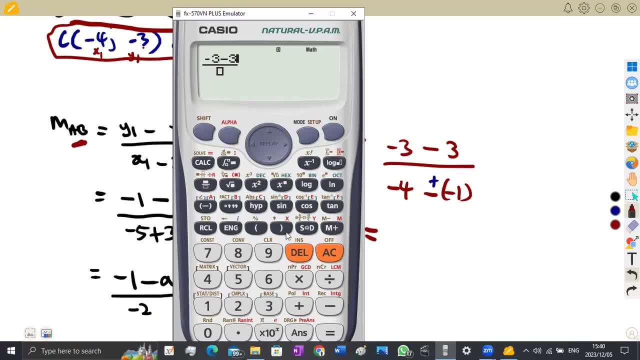 So this is minus 3, minus 3, like this, over minus 4, like this. Then you subtract. What are we subtracting? Minus 1.. So just open a bracket and press minus 1, like this: So this is going to give you a 2.. 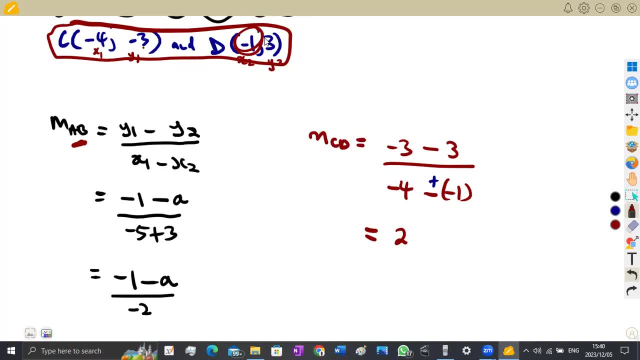 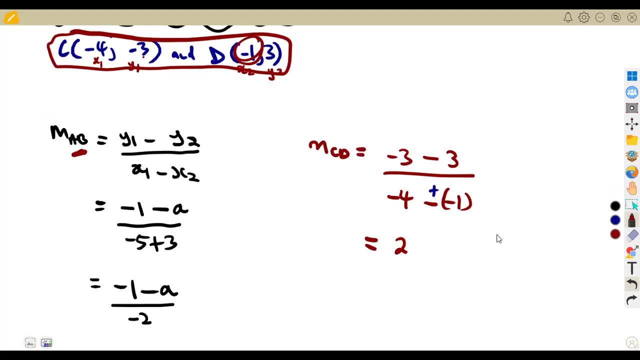 So we are obtaining the gradient, which is the numerical. numerical, That is a number, not in terms of X, or in terms of A, or in terms of what. No, you're getting a number, a direct number, an exact value. 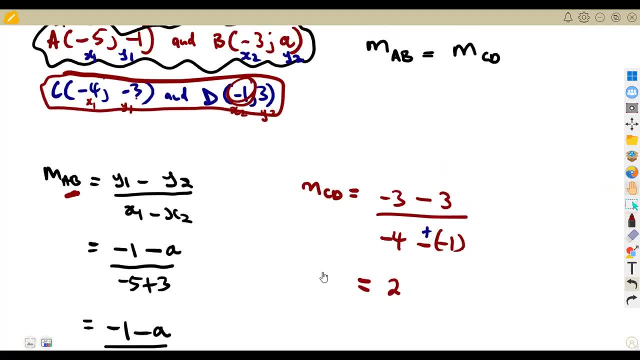 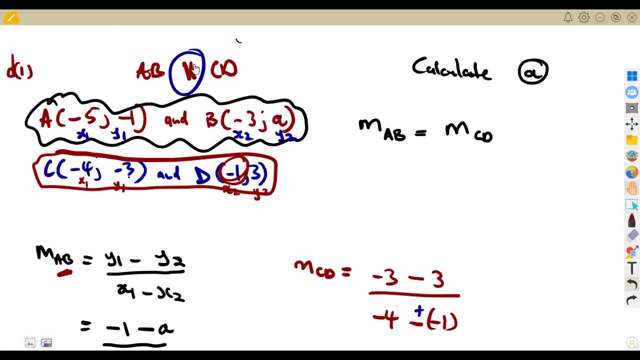 All right, Now that we have got our gradients, let's go to the condition. The condition was saying: These two lines, they are what They are parallel. AB is parallel to CD, AB is parallel parallel. So if they are parallel, we said they have what? 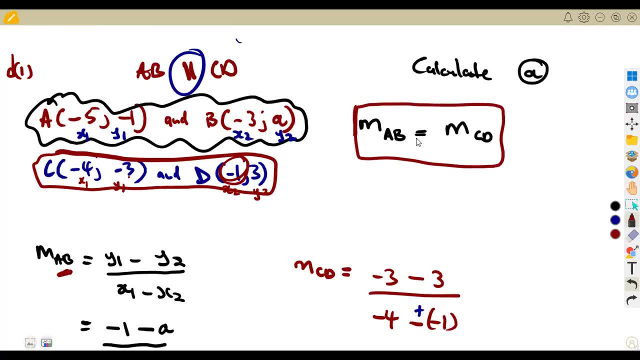 Same gradient. The gradient of AB must be equal to the gradient of CD. We are told that they are parallel, As we know that if two lines are parallel they have same gradient. So that is the condition that you're going to use. 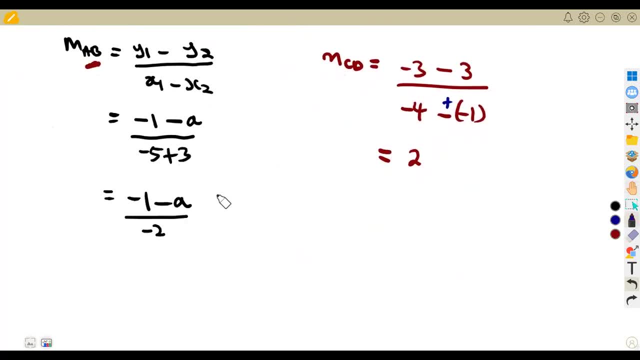 Because they are what They are: parallel. So you're going to tell yourself that since these two lines are parallel, and I know that the gradient of line AB is equal to the gradient of CD, I'm going to form an equation from there. 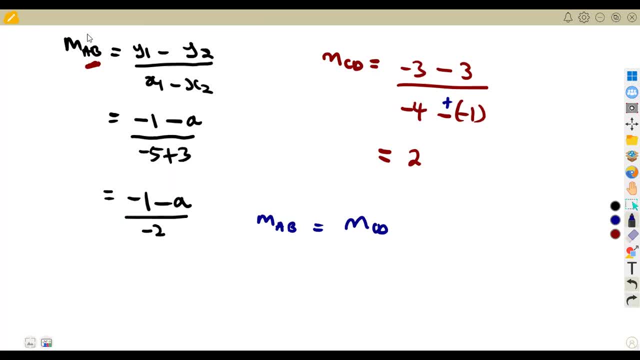 It's an equation, because I have the gradient of what? Of the line AB, which is minus 1, minus A over minus 2, which is equal to the gradient of CD. I have the CD, which is 2.. So remember, I told you guys. 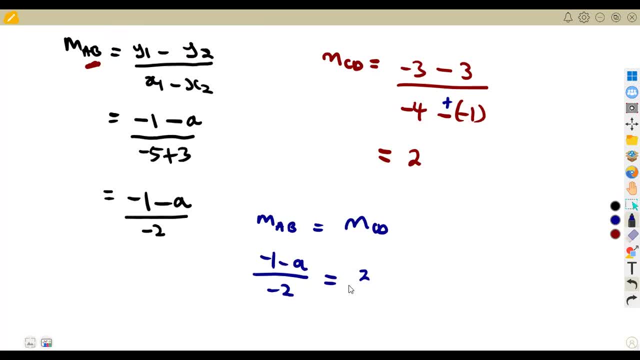 Every whole number can be written as a fraction. at the moment we write it as over 1. So that you can be able to solve for A. So from this we can solve for A. Remember, the question was for us to find or to calculate the value of A. 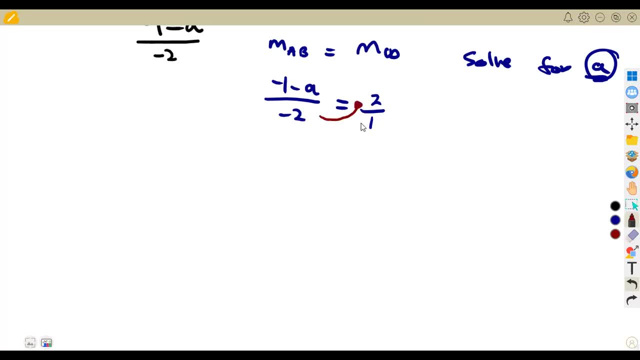 So we're going to solve, since this is now an equation. So remember: you can cross, multiply to remove your fractions. So that's 1 times negative 1, which is negative 1.. 1 times negative A, which is negative A, is equal to negative 2.. 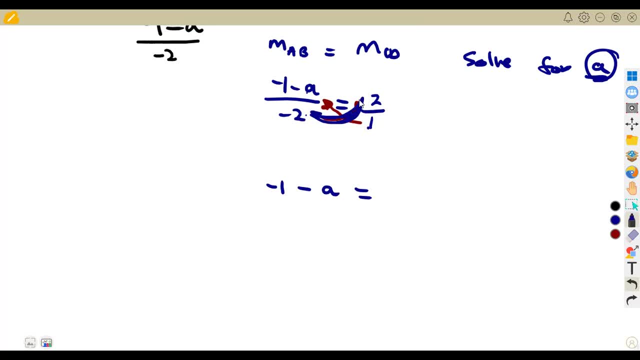 2 times negative 2.. You're multiplying these two cross like this over the equal sign. So minus 2 times 2, that's a minus 4.. All right, So to find A. we can transpose this to the other side. 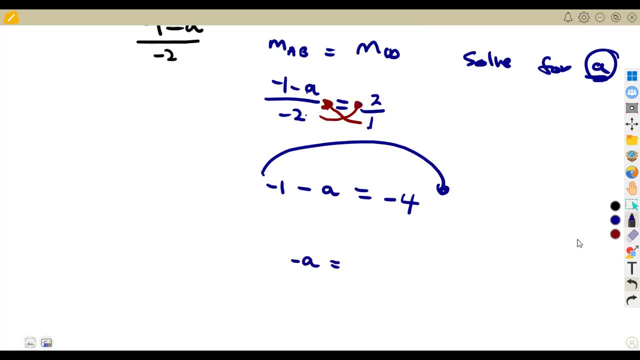 It becomes a positive there, So it's going to be: minus A is equal to minus 4 plus 1.. It was a negative, So it's going to be a positive, And minus 4 plus 1 from our calculator is going to give us negative 3.. 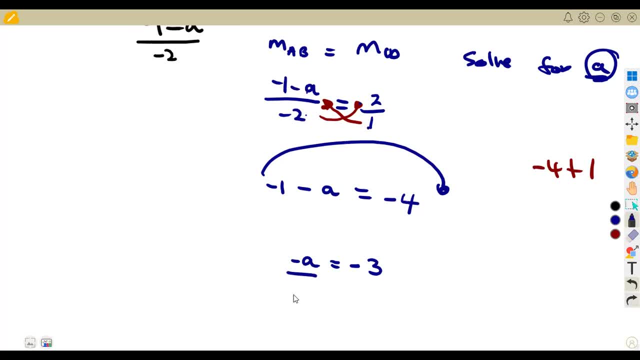 So if we divide by negative 2, we remove this negative on A, We divide by negative 1 so that this will cancel, because minus A simply means minus 1A, So minus 1 and minus 1 cancels. So A is going to be equal to what? 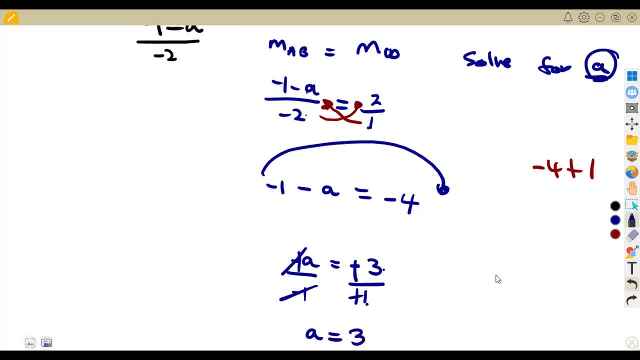 1 into 3.. That's going to be a positive 3 in that manner, So meaning to say we are going to obtain the value of A as a what As a 3.. The moment we put this A here as a 3,. 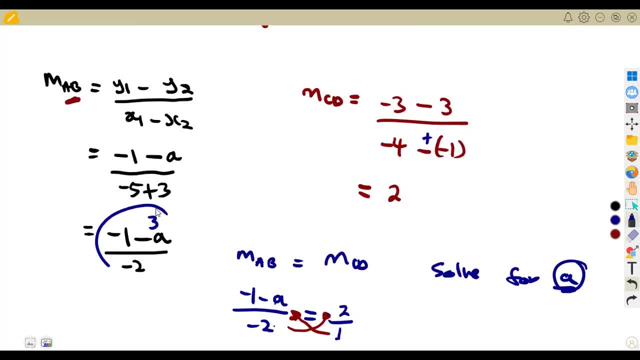 the moment we put A here as a 3,, we are going to see that our gradient is going to be equal to 2.. And that is to show that this is the exact value of A And because we said they are parallel. 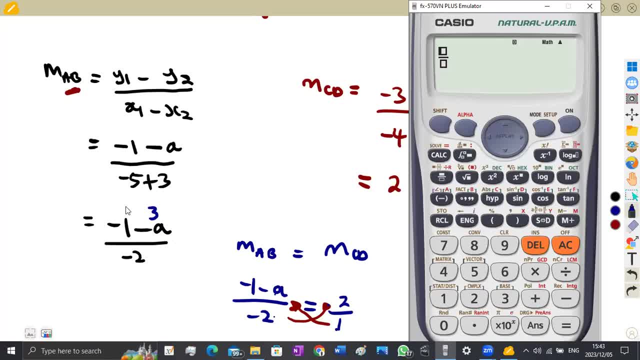 so they must have the same gradient. So let's put our calculator and see We said A is 3.. So in place of A let's put 3.. So this is minus 1 minus 3, okay, Over minus 2.. 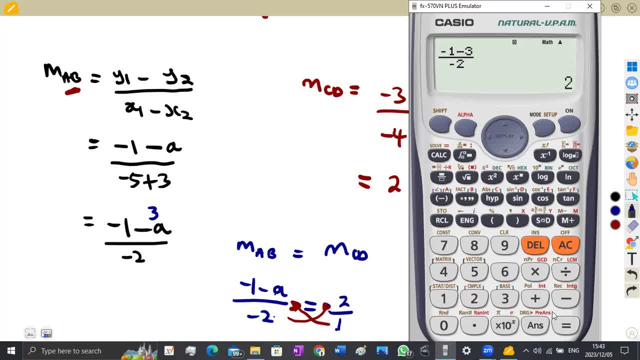 So you divide by what? By negative 2, like this, And this gives us a positive 2.. So it means, if we have got a gradient of 2, and here we have got a gradient of 2, what does it mean? 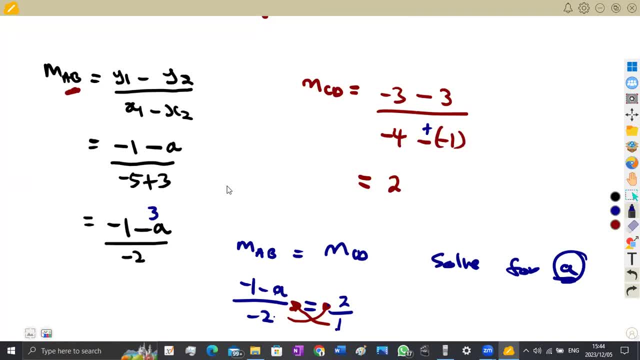 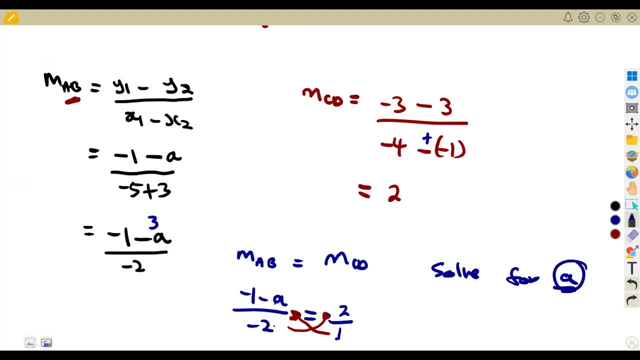 These two lines. they are what. They are: parallel to each other. because we said parallel lines, you have got same or equal gradients. So that was the idea of this question, This is how you are going to answer these questions, and so on. 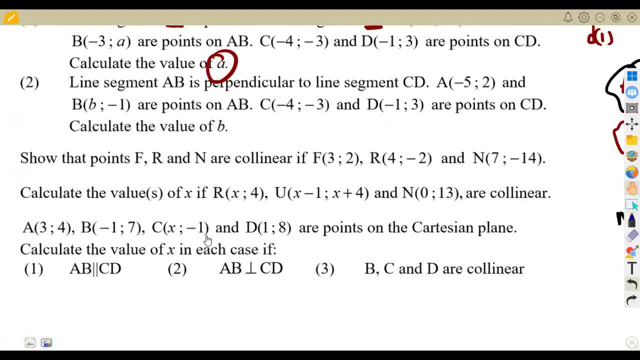 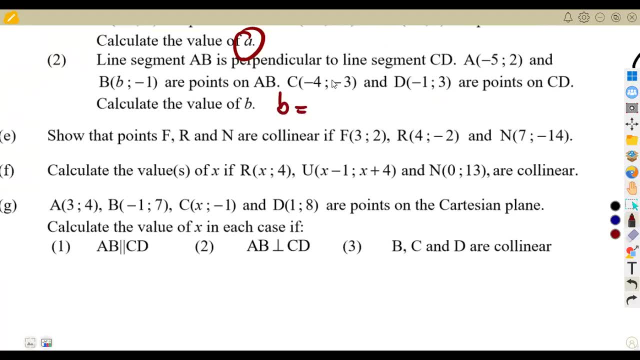 So it is the same thing If they are perpendicular. I want you to try that and see how you can calculate the value of B. So if you calculate properly here, the value of B was going to give you 1. If they are perpendicular: 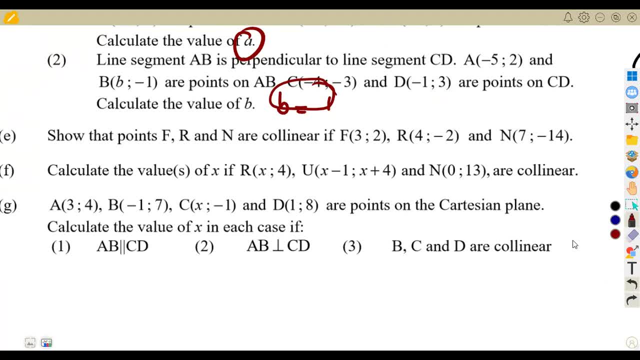 remember I said, if they are perpendicular, you multiply what, You multiply the gradients. So you are going to multiply the gradient of the first line times the gradient of the second line. It must give you what A negative 1.. So I want you to try. 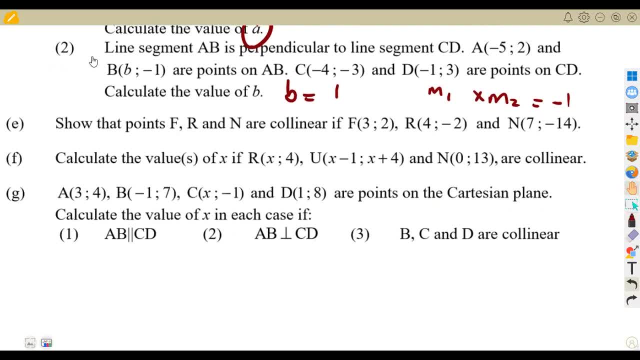 but if it gives you a challenge, let me know about this person so that we can work with it. We can work with this person together in our next class. Okay, Let us see the other part, which is E On E. we are given. 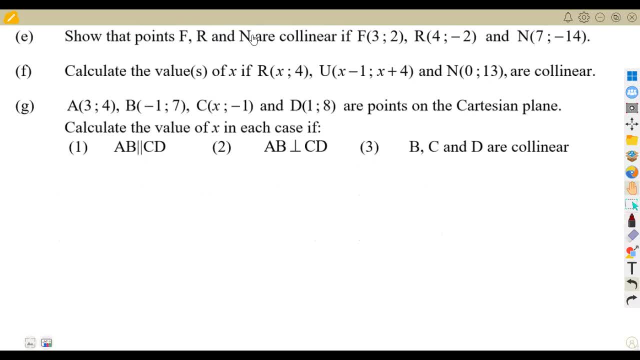 show that the points F, R and N are collinear. We are back to that statement that I talked about the collinear concept. All right, So on the collinear concept, we said we must have the same gradient. So what you can simply do, 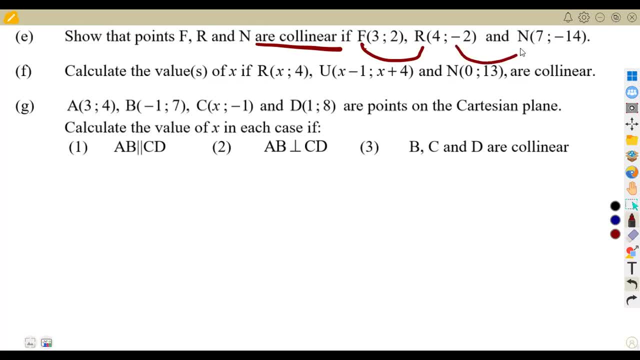 you can calculate the gradient of F, R and you can calculate the gradient of what? Of R, N, just like that, All right. So let us see the collinear concept. Think about equal gradients, Equal, equal, equal. 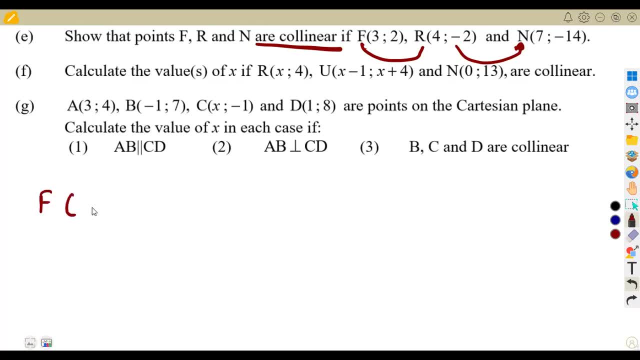 Okay, So let us start with F and R. The point F is 3,, 2 is given and the point R is given as 4, negative 2.. So I want you to use these two points, Calculate the gradient. 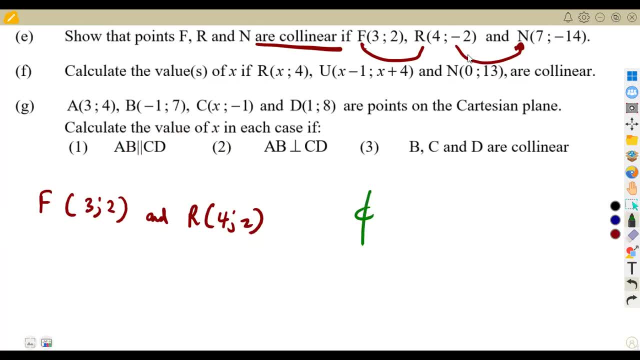 Okay, You do the same thing on R and N, R, N, like that. Just take the next two. or even take T, F, N, It is one and the same thing. So you can just take R, which is 4, negative 2.. 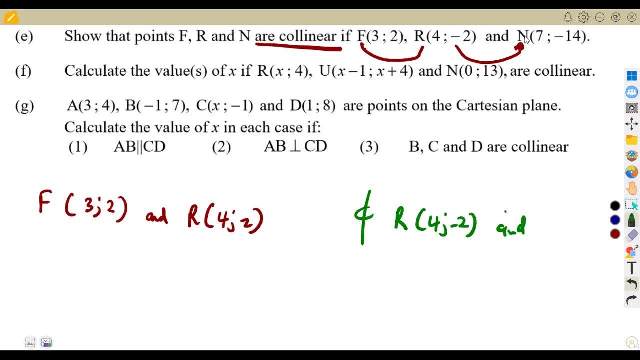 And in this case you're going to take the point N, which is 7, negative 14,, like that. So that's it. So we show that To show is like to prove. We are asked to show that these two lines: 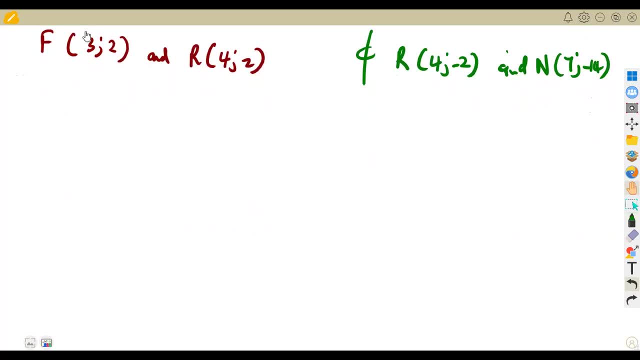 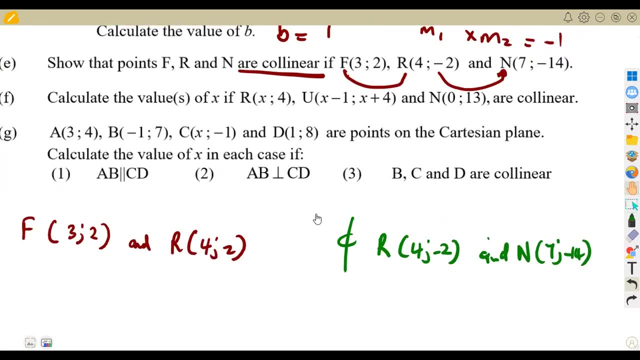 I mean the points F, R and N are collinear, They're only straight lines. Why am I? Why am I having 4, minus 2, and the other one was 4?? Oh, this is 4, negative 2.. 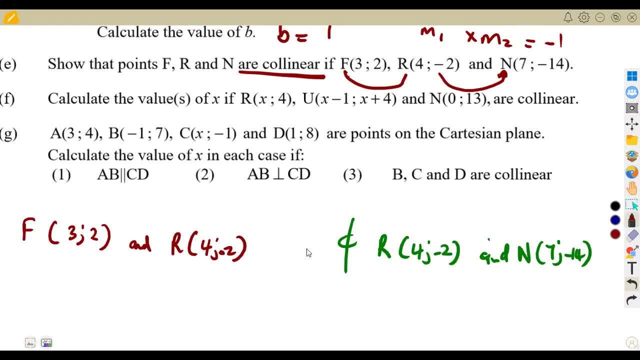 Check note: This is 4, negative 2.. I'm even surprised to say: why am I having a negative and here it's a positive? This is 4, minus 2, the point R, The point F, is 3, 2.. 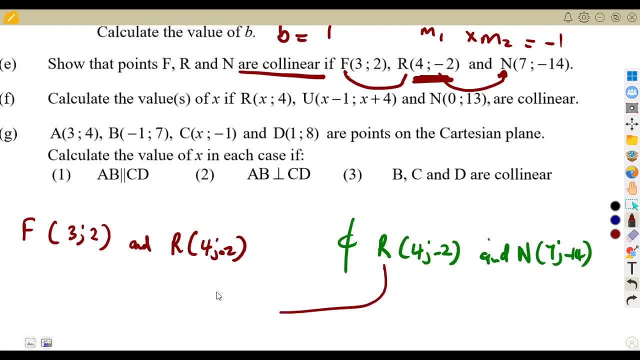 R 4, minus 2, which is the same R that we have. This one is the same point. we just separated to say: let's use R here. The same R that we use is the same R that we are using. 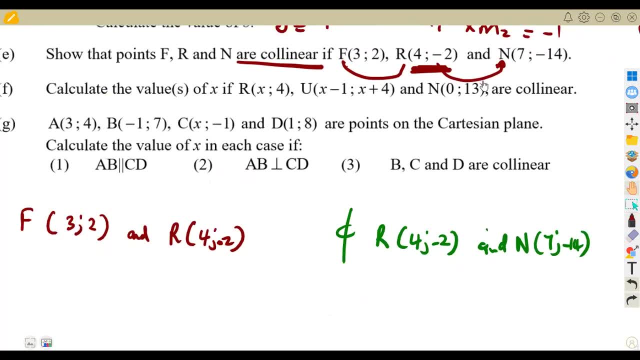 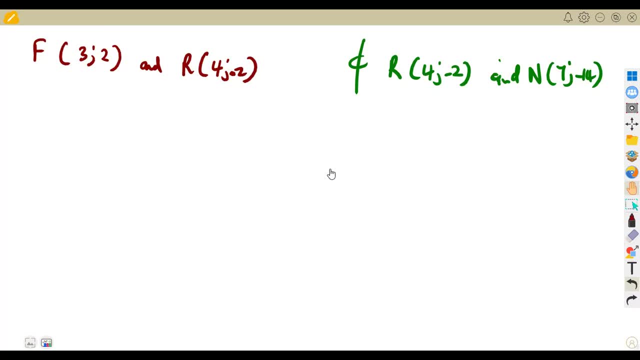 It's one and the same thing, you see. So They must have same gradient, these lines, if truly we are, I mean the points between F and R, between R and N- we must obtain the same gradient. So let's calculate the gradient. 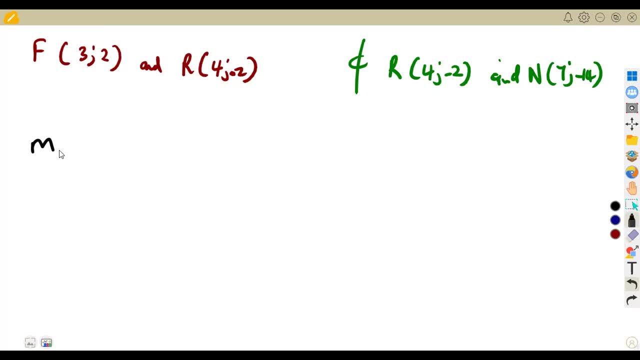 The gradient of FR. All right, so the gradient M. So the gradient of FR is just going to be changing Y over the change in X. So that's it. This is our first point. This will be our second point. So we're just going to have Y1, minus Y2,. 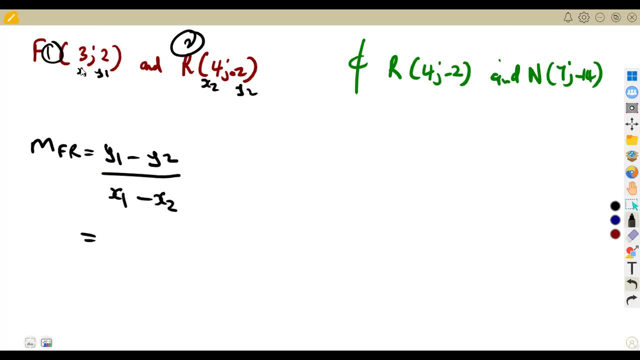 over X1, minus X2.. So let's substitute Y1.. Here it's a 2. The Y value from the first point minus the Y value from the second point, which is a minus 2. So that's minus minus, which gives us what. 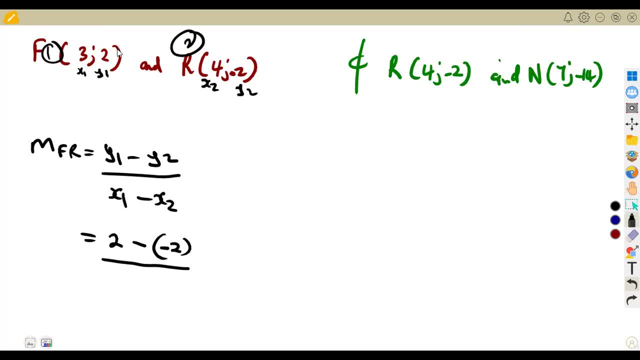 A positive- We'll just leave it like that- Over X1, which is a 3. So that's 3, minus X2.. The X value from the first point, from the second point, that's X2, sorry. 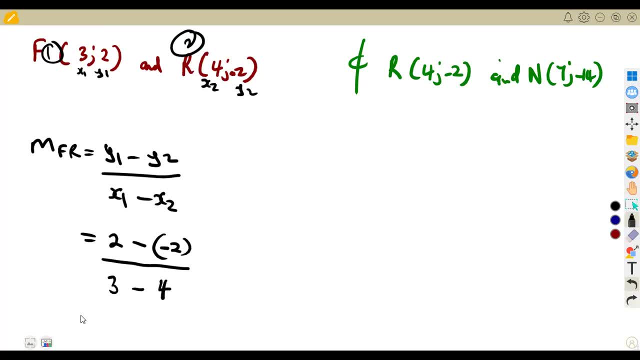 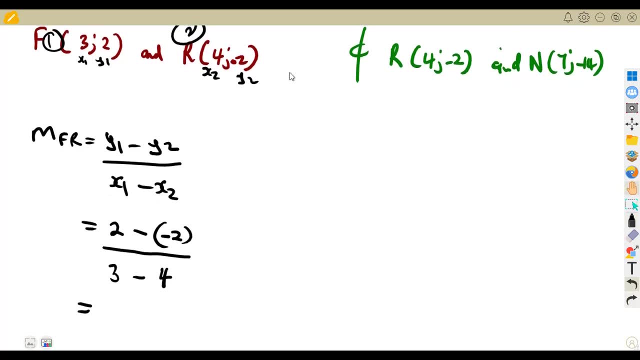 from the second point, which is a 4.. So, So this can be simplified, like I say, direct on our calculators. We can simplify this All right. so this is the condition of the collinear concept. Let's see 2.. 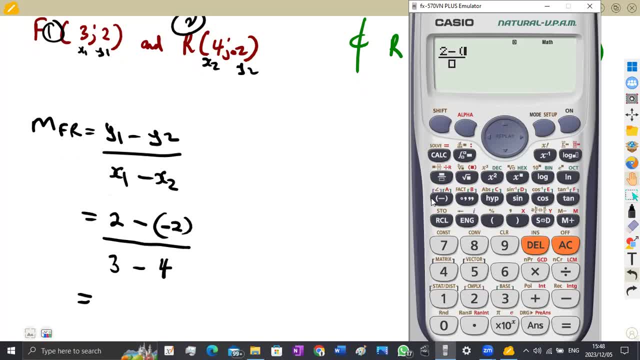 We subtract. What are we subtracting? Minus 2.. So just open a bracket for that negative 2, okay, Over 3, minus 4.. So this is 3, minus 4, like this, It's just going to give us okay. 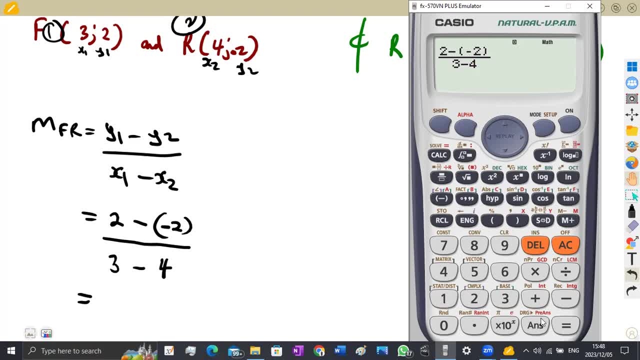 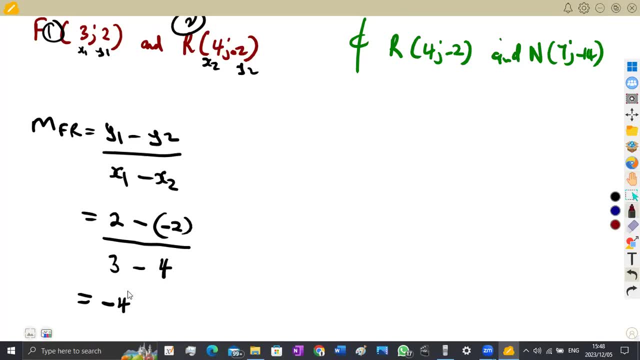 This is what: 4 over negative 1,, which is negative 4.. So this is going to give us a negative 4,. okay, That's it, A negative 4.. So we are obtaining a negative 4 from FR. 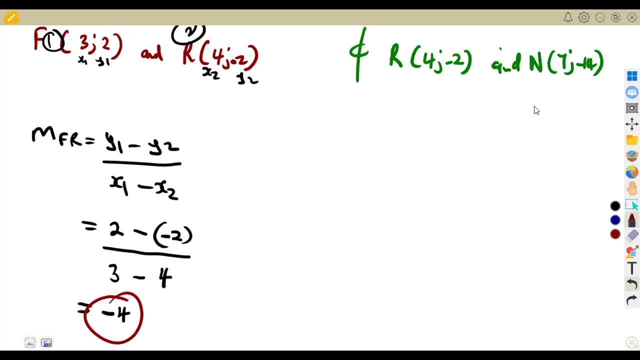 If so, if truly they are collinear, we must give the same answer: Okay, let's check, Let's check, let's check RN. So this is going to be the gradient of RN, The change in Y over the change in X. again, 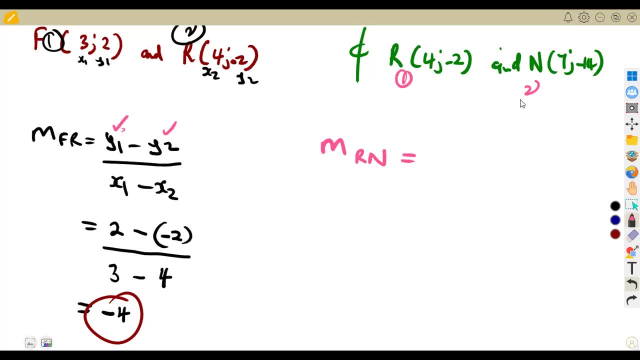 that's Y1 minus Y2.. So this is our first point. our second point: We're just going to have X1.. Y1. This can be your Y1, Y2, in an order that you want. okay, Y1, that is minus 2, minus Y2, Y1, minus Y2.. 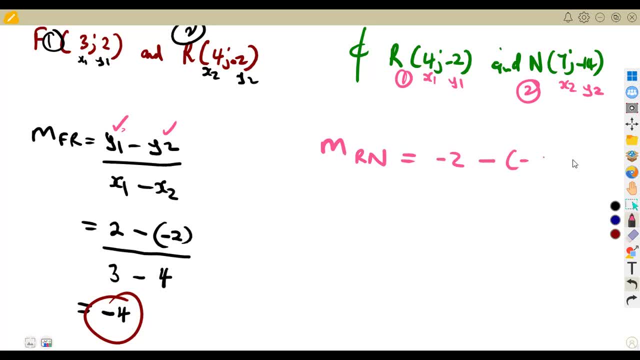 Y2 carries a negative, So that's a negative 14, all right Over X1 minus X2.. X1, that's a 4, minus X2.. X2, which is a 7.. So this is going to give us the gradient. 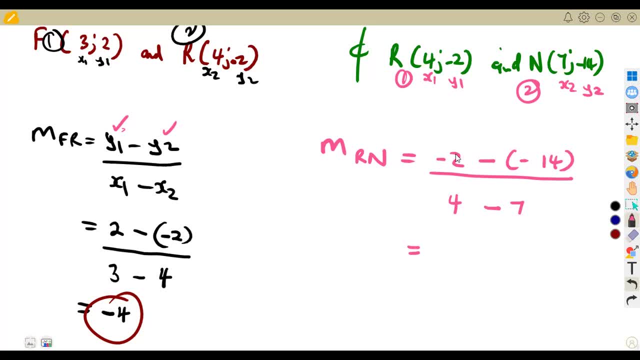 I have the same thing here. Why is it? I'm doubting There is big values, but do not doubt the answers, guys. Like do not doubt your calculations, all right In XM, but there are big values there. 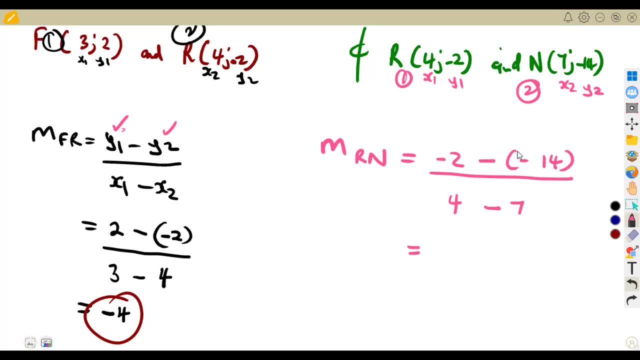 which is one and the same thing, Minus 2, minus, we subtract. What are we subtracting? Minus 14.. Put a bracket minus 14 like that Over 4 minus 7.. So this is 4 minus a 7, like this: 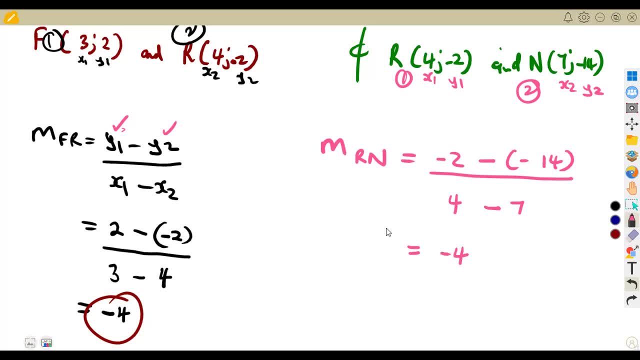 which is going to give us a negative 4, a negative 4.. So we have got the same gradient there. Okay, guys, I did not show you the calculator, Sorry for that. This is it. This is it like this: minus 2,, minus minus. 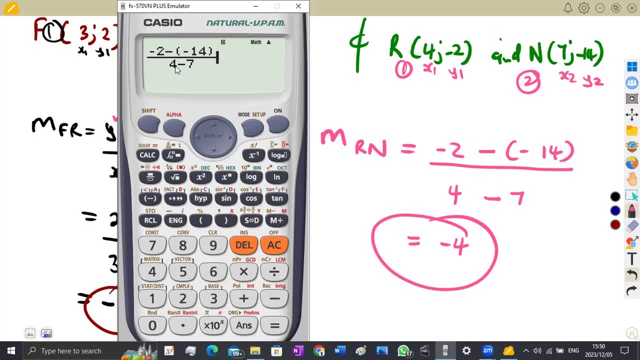 Okay, so let's condition minus 2,, minus 14, then over 4, minus 3.. And this is equal to what? Negative 4.. So that can be like that. So meaning to say, guys, as you can see, these two gradients are the same. 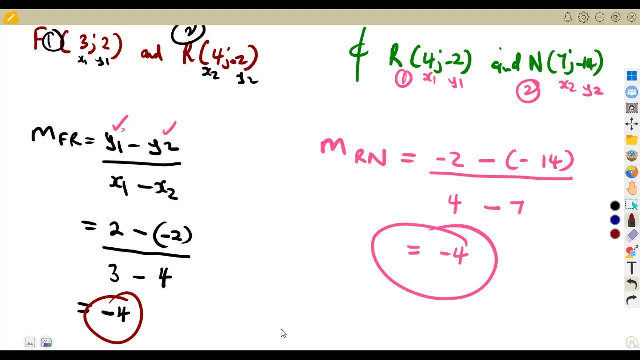 So therefore, these points are collinear. So therefore, F, R And the point N are collinear. All right, They are collinear, We have got the same gradient. So that's the idea of being what Collinear. 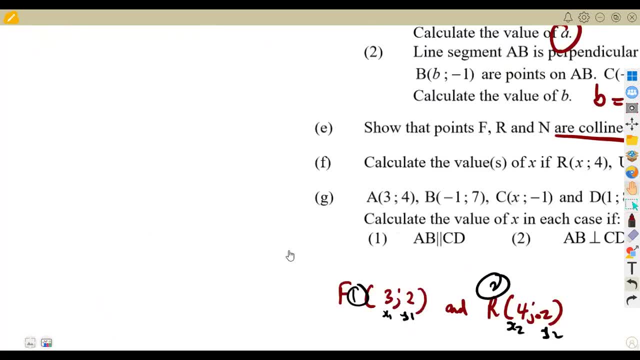 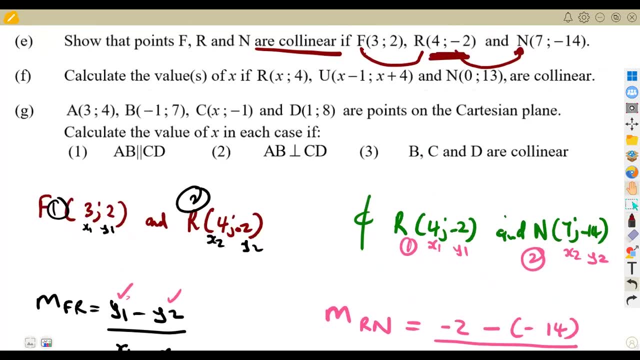 I hope we are together, guys, All right. So questions can be like that And just have to be careful on your attempting of the questions. So there are so many questions, guys, I'm not going to answer all of these questions with you. 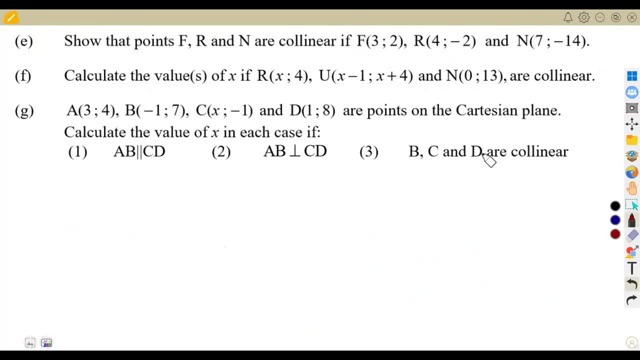 Hey, what points on the Cartesian? Calculate the value of X in each case if these are collinear. So you're just going to use those ideas that we've been talking about of the collinear concept and so forth and so forth, And on this one, on F, we are given: calculate the values of X. 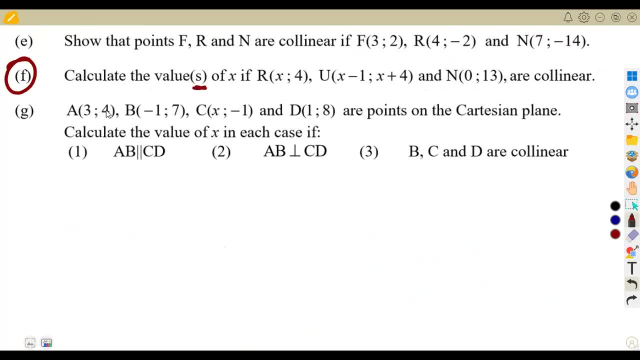 They're saying the value of values. Calculate the value or values, which means they can be many. They can be two possible values. Okay, Anyways, let's try if these points are collinear, So I'm going to attempt this. 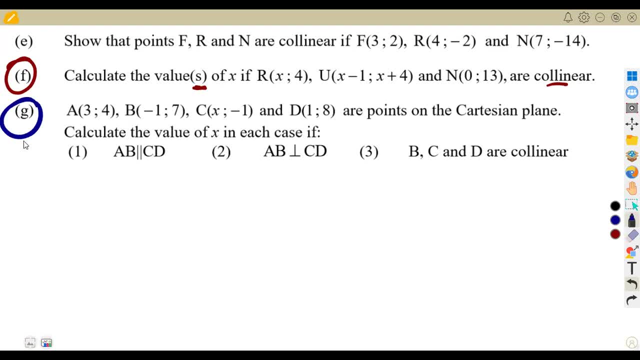 Then you guys are going to attempt G, Try to attempt the question G. Please do that and let me know, on the comment section, the answers that you're going to get for X, for these questions that you're going to answer from one, two and so forth. 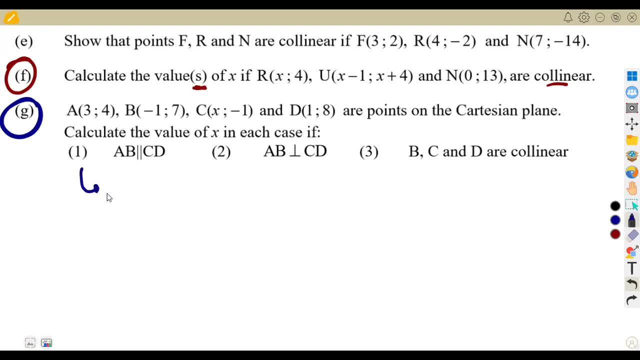 But if you're to calculate properly this one, for the first one I'm just going to give you the answers, But I want you to try and see if you're getting these answers that I'm giving you here, Because I did calculate this. 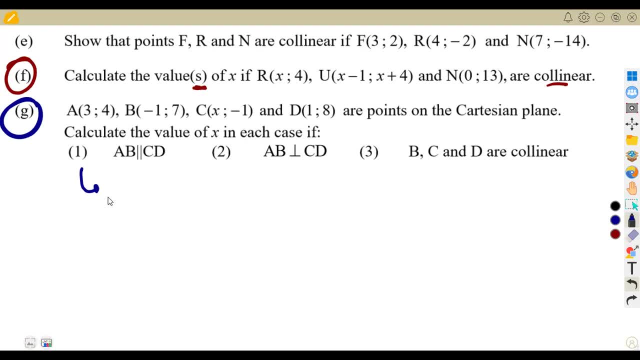 On my revision when I was just like: let me see these persons. So this was: X is equal to 18.. And here you're going to get your X being equal to negative 23 over four, All right. And this you're going to have your X as a negative 17.. 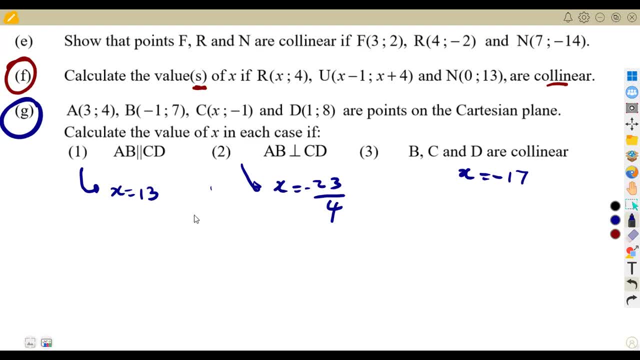 So, like I said, if you have a challenge in this, let me know so that you can do this question together in our next class. But for now I'm just going to answer with you question G. All right, I'm just going. 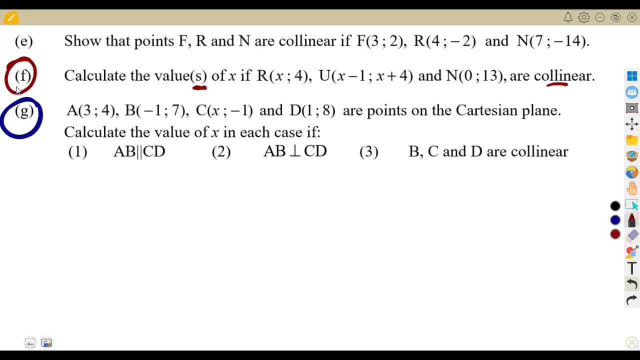 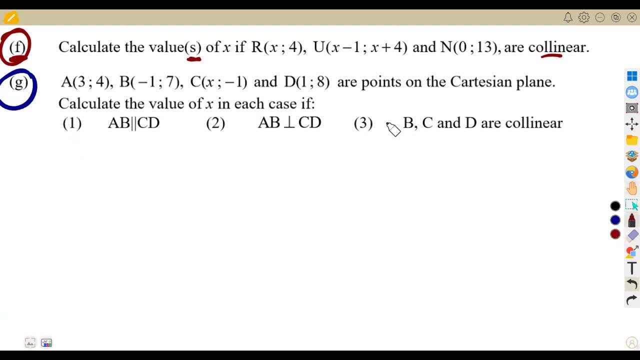 To do with you here the G part, I mean the F, So the F part. calculate the value of values. Like I said, they can be two possible values or it's just a single value that you have. All right, If these are U and N are collinear. 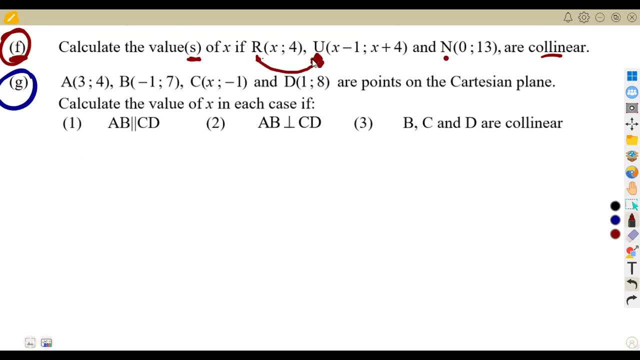 So I said if they are collinear I can use the two points, R and U, to calculate the gradient, Then U and what N to calculate the gradient. All right, So that means the gradient of R- U must be equal To the gradient of what? U. and the previous case we were to show that they are collinear. 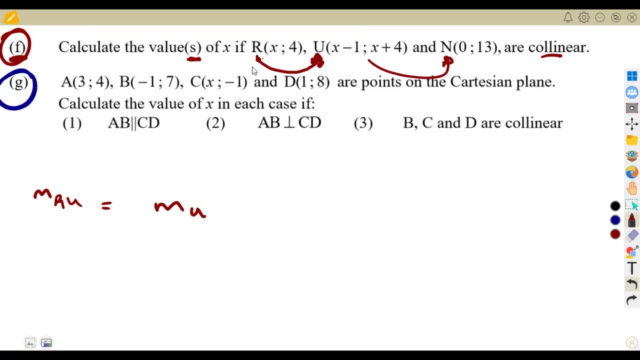 It is you who has to show that. Now you're not showing. You're not showing. You're already told that they are collinear. So you're actually writing that this gradient must be equal to this. Already you're told that. You're told they're collinear. 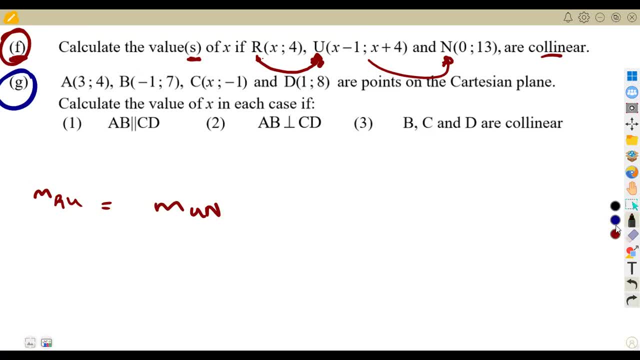 And this is the condition of being collinear, The gradients should be the same, All right, So let's calculate the gradient of R? U, The gradient of R? U from the change in Y over the change in X, Y1 minus Y2 over X1 minus X2.. 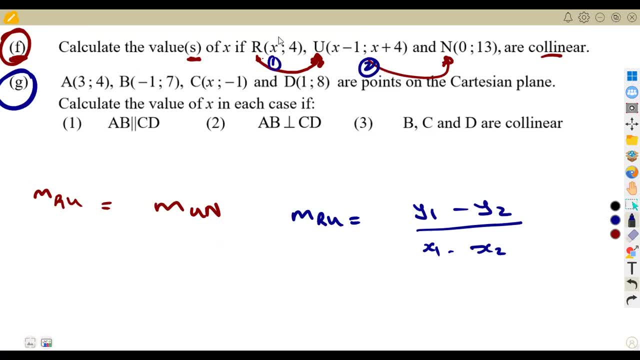 This is going to be our first point And this will be our second point. So this is X1, Y1, X2, Y2.. This is your choice, Okay, So Y1,, that's a 4.. So 4 minus Y2.. 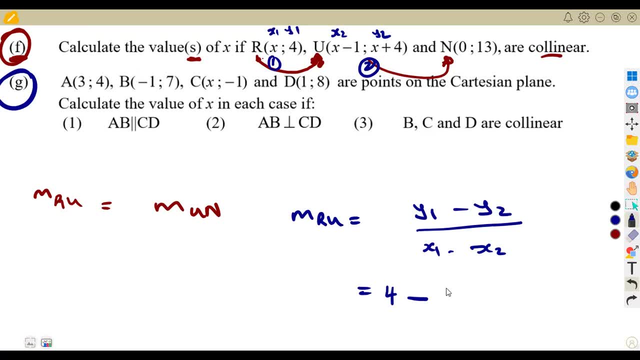 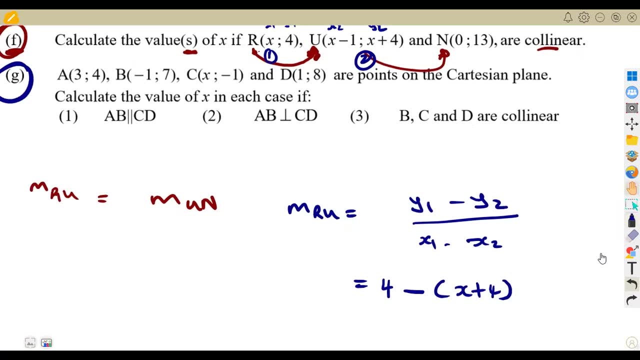 Y2. on this side, Y2 is X plus 4.. So just open a bracket, Since this is the whole of this part. Yes, To be affected by a negative since you're subtracting, All right, So let's move on to X1 minus X2.. 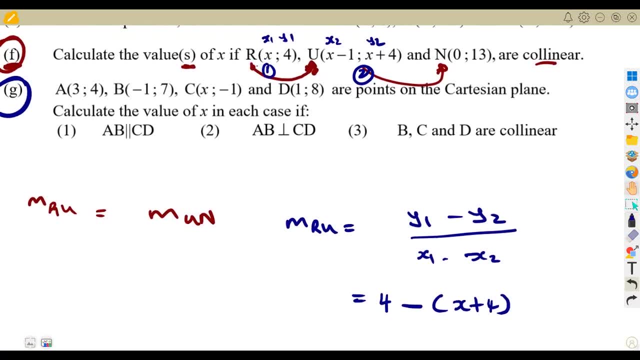 The X value is X on X1.. All right, That's over X1, which is X minus X2.. X2 here is X minus 1.. So again open a bracket X minus 1, like that. So you're going to substitute X1 minus X2.. 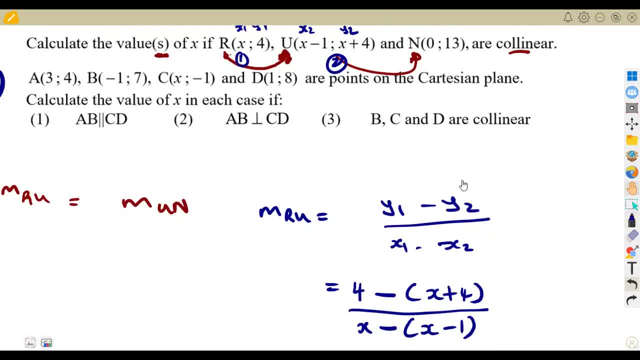 That's your X1.. This is your X2.. All right, You do that. You simplify if you want. Yes, you can just simplify. You're going to do. You're going to do the same thing on your end. Let's just simplify. RAU first. 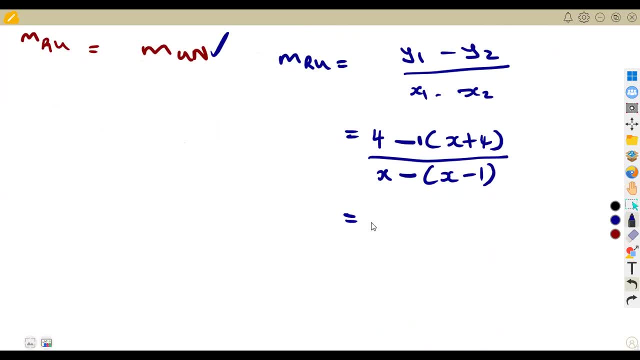 So let's affect everything. Distribute by negative 1 throughout, This is going to be 4.. Negative 1 multiplies X. Negative 1 multiplies 4.. So what are we going to get? Negative 1 times X. 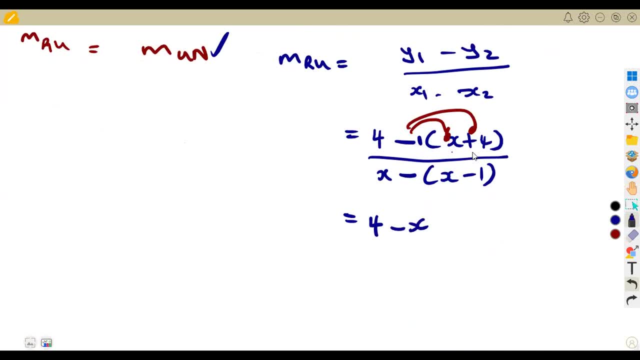 That's negative. X Negative 1 times a plus 4. A plus A plus A plus: It gives us a negative 4. A minus and a plus, That's a negative. All right, Everything over. We simplify this side. 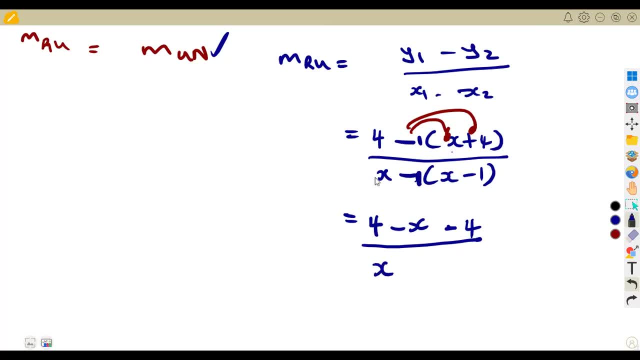 Again, we distribute: This is a negative 1.. So this is going to be X, Then negative 1 times X here. All right, What are we going to get? That's the negative X. Okay, Let me just change this. 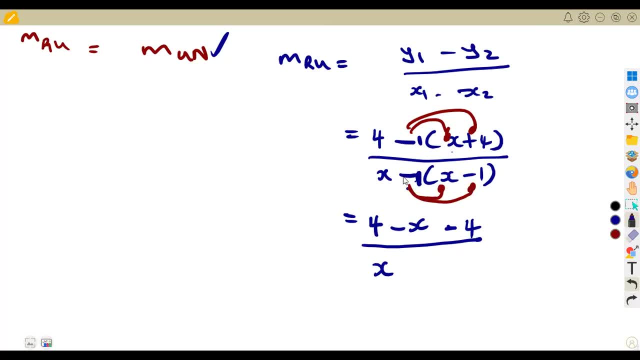 Negative 1 multiplies X. Negative 1 multiplies negative 1.. All right, Take note, This is negative 1.. Not a 7,, but negative 1.. Negative 1 like this. Let me just try and put this way: 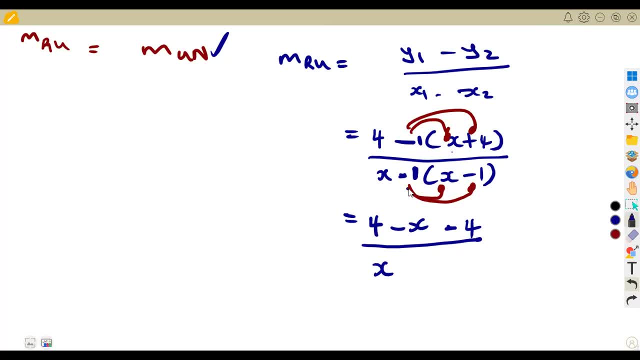 Negative 1, like this: Okay, So what are we going to have here? Negative 1 times X, which is negative, X Negative 1 times a negative 1.. Negative, negative, negative, negative- It's a positive. Whenever you multiply this, you get a positive. 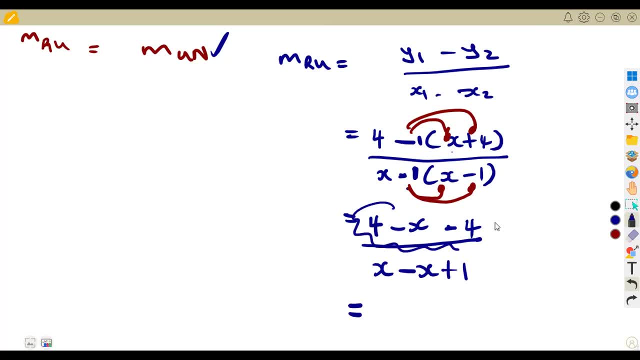 So you can be able to simplify from the numerator. We've got like terms that you can simplify for minus 4, which is a 0. So 4 minus 4, like this, it gives us a 0. So you are left with what? 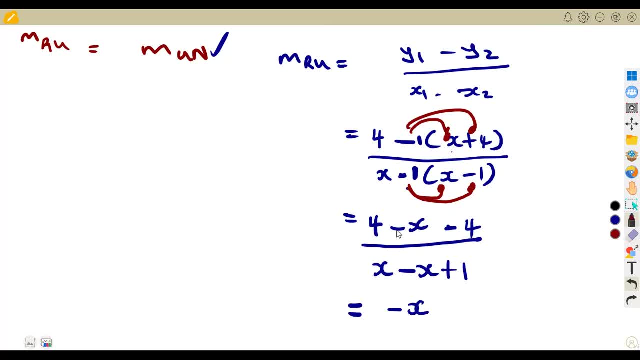 With minus X. So that will be minus X, because this is cancel. This one is this one. Okay, So you remain with minus X. All right, Over The same thing here: The X and the X. as you can see, it cancels X minus X. 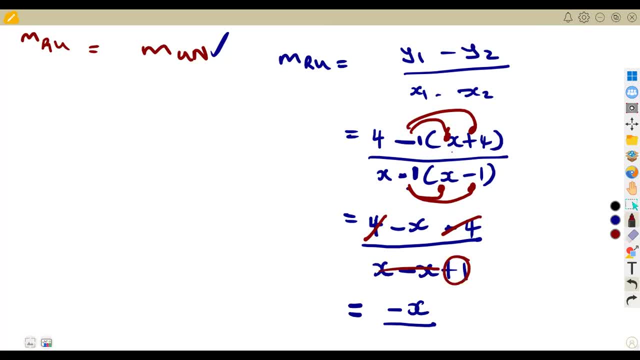 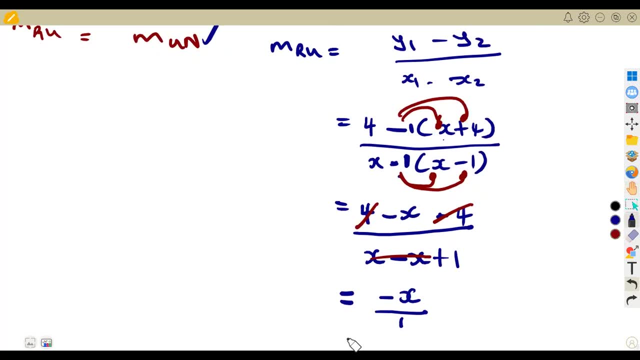 That's a 0.. So this one and this one cancels, remain with what A 1.. And guys, 1, I mean minus X over 1 is just minus X. So this one is just a minus X, Just like minus 5 divided by 1 is a minus 5.. 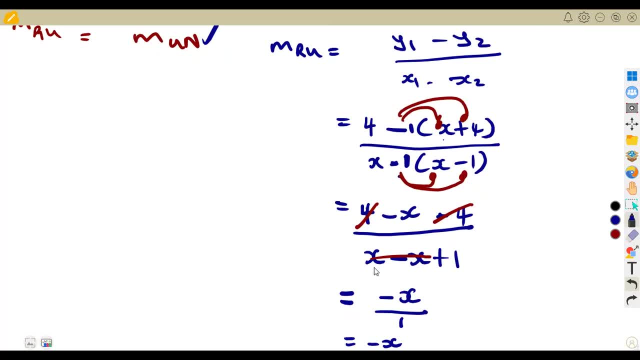 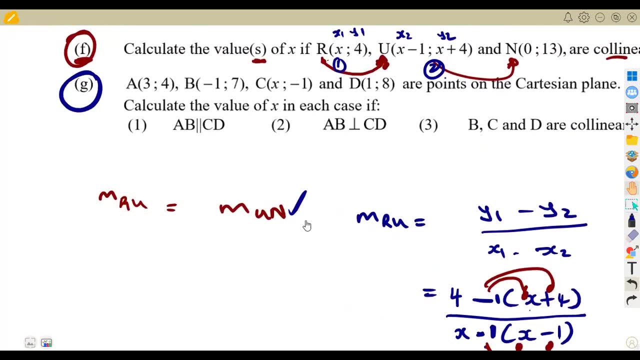 Or any number divided by 1, it remains as it is. We know that. Okay, We talked about this. Okay, We talked about this. Let's move on To the other point. Now we're going to use U R U N U N. 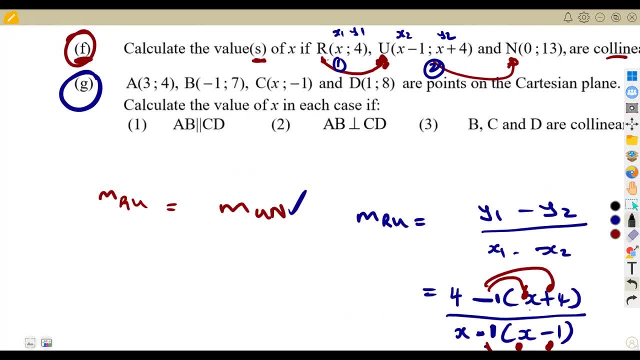 We used R U, Then we use U- N, From U to N. This is what you're going to need this time, So it means this is no longer like valid. We are not going to have another thing to consider, Just like U. this is. we now consider U N like this: 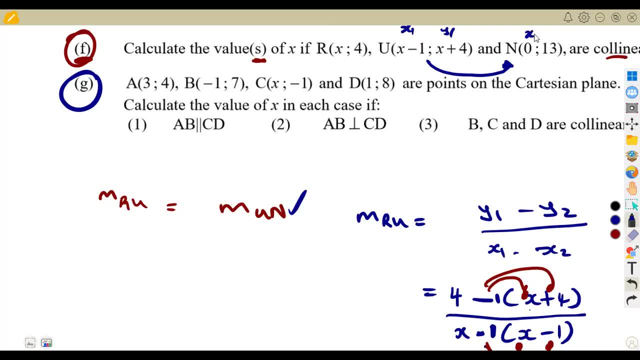 So this is going to be our X1, Y1.. This is going to be our X2, Y2.. All right, So let's consider, Let's consider our gradients. So the gradient of U- N in that manner is going to be from the formula Y1 minus Y2.. 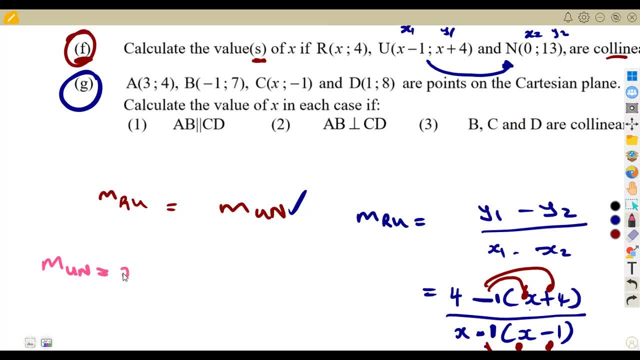 It does not change. So Y1 here is X plus 4.. So this is X plus 4 minus Y2.. Y2, the Y value from the second point is a 13.. So 13 is just a normal number. There is nothing to open a bracket. 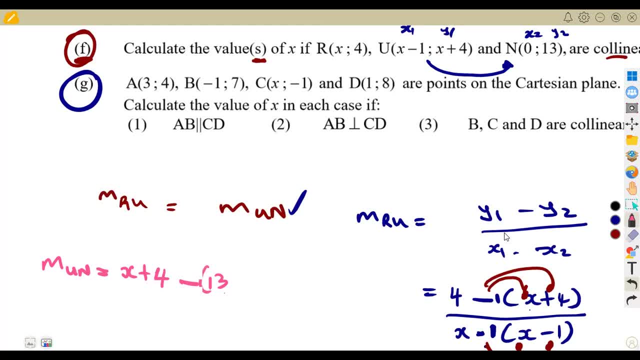 It's just a direct. If you want, you could have opened a bracket like that. Whatever that you're subtracting, it's good for you to open a bracket So that you understand that that one is a single term, So the bracket is not that important when it is like that. 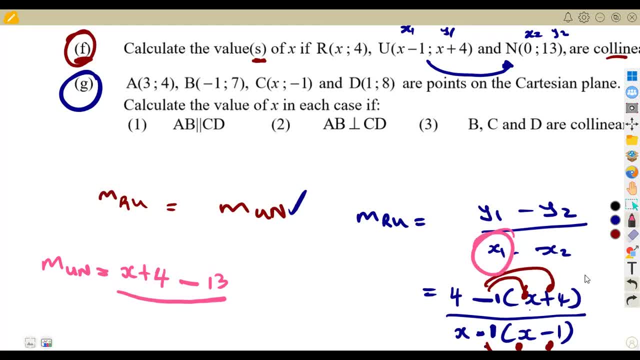 All right Over X1 minus X2.. So you're going to need the idea of X1 minus X2.. So X1 here is X minus 1.. So it's X minus 1, which is going to sub. The algebraic expression is the one that is subtracting a term. 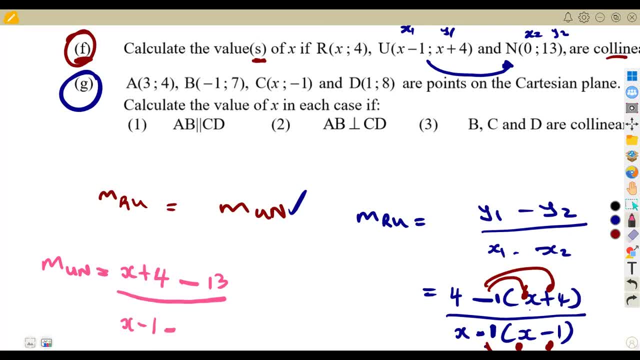 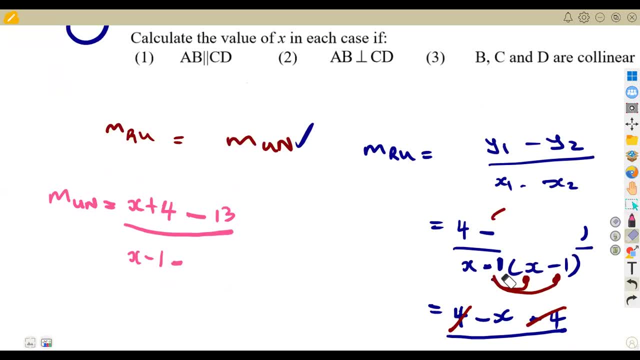 All right. So there is no need for you to have this in a bracket, Unless you are subtracting It like this. but we were subtracting. we have to subtract every part here, So that part that we are supposed to subtract guys is supposed to be in a bracket. 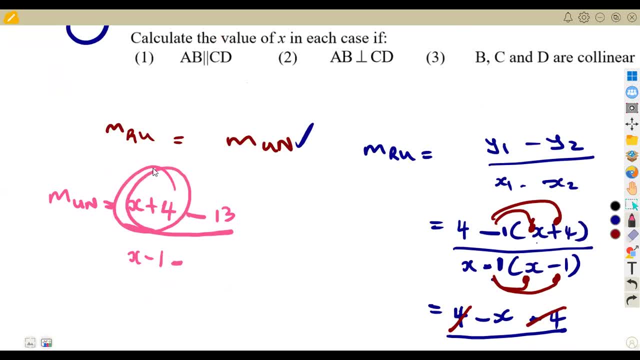 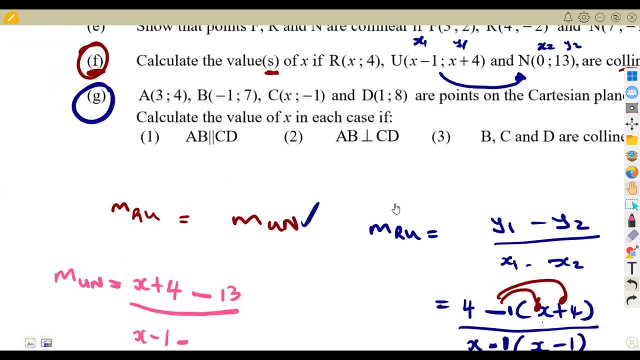 The part that you're supposed to subtract. here. we are not subtracting X plus four. It is X plus four which is going to subtract this 18.. So there's no need for you to write even that 18 in the inside of bracket. 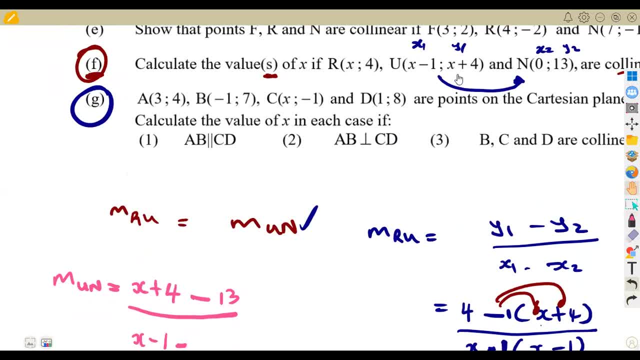 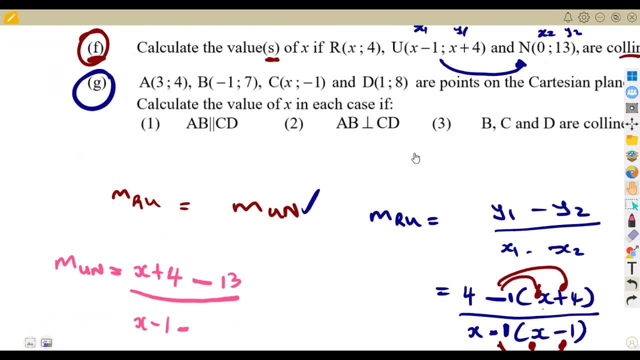 All right. So here we're saying X1, which is, uh, here, X minus four. That's our X1. X minus one, Yeah, Minus X2.. Our X2.. X2 data is zero, So you're going to subtract, and zero subtracting is zero, guys, simply means there's nothing that you're subtracting there. 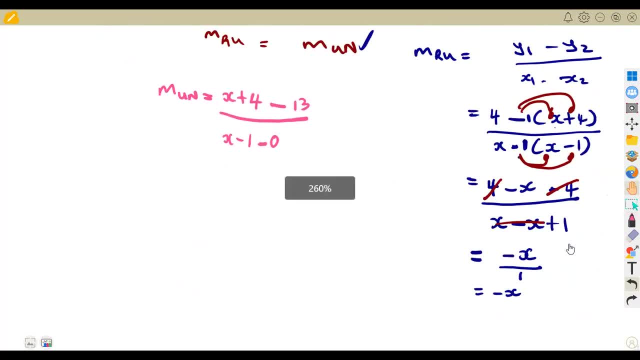 All right, Anyway, this is what we're going to have at the end. So now we can be able to simplify this here. So this is the gradient of UN. Uh, so that'll be X four minus 18, which is a negative nine four minus 18.. 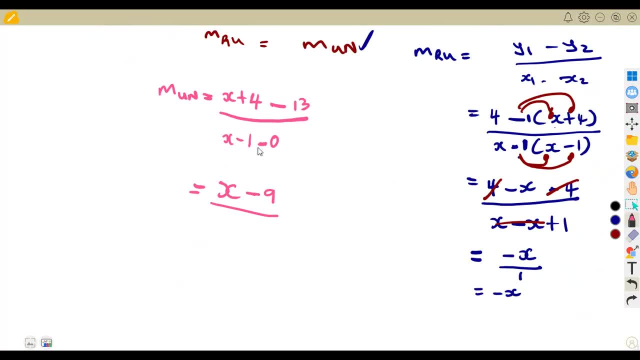 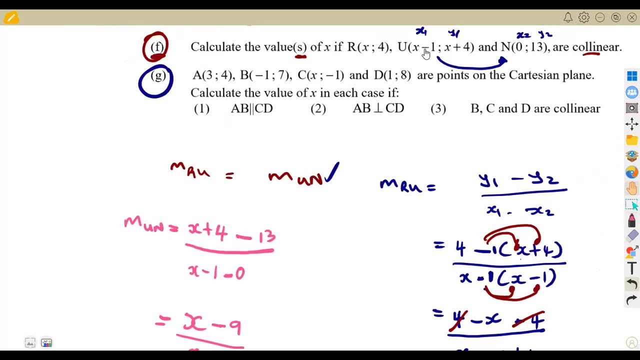 That's a negative nine over X minus one. That's minus one minus zero, which is just X minus one. Okay, That's just X minus one. Then there's nothing that you're going to do in this case, There's nothing that you can simplify, because it's just X minus one and there's a minus zero. 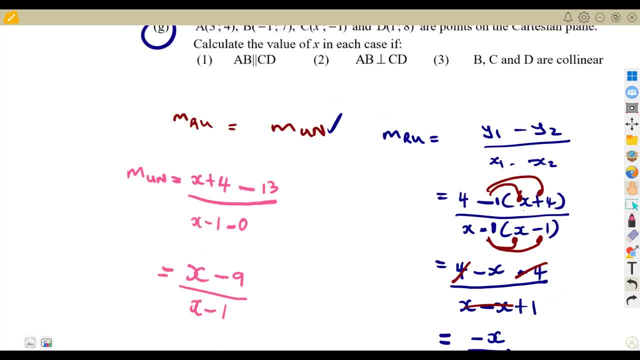 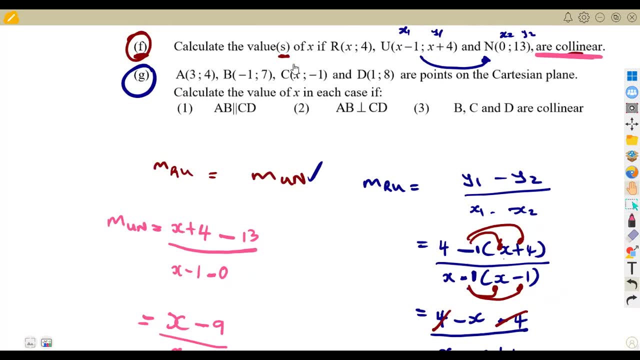 So that is just going to remain as what is X minus one. But remember our condition that, we are told, is that these lines, these points, are four linear. So if the points are four linear, how can we find now the value, or the values of X? was you're supposed to calculate? for what? 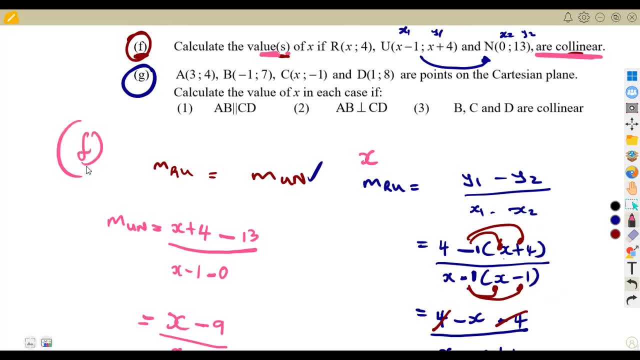 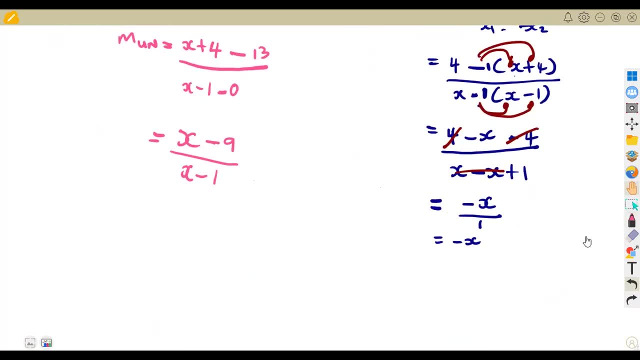 For the value of X. this is the value that we are supposed to To be calculating. So how can we calculate for X? Now we have to consider the idea that we talked about. If these two, uh, if these three points are four linear, their gradients is going to be the same. 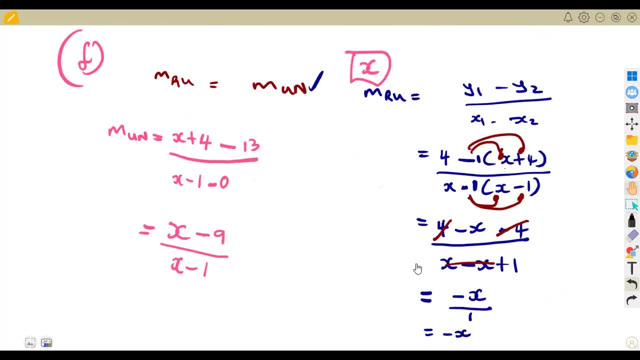 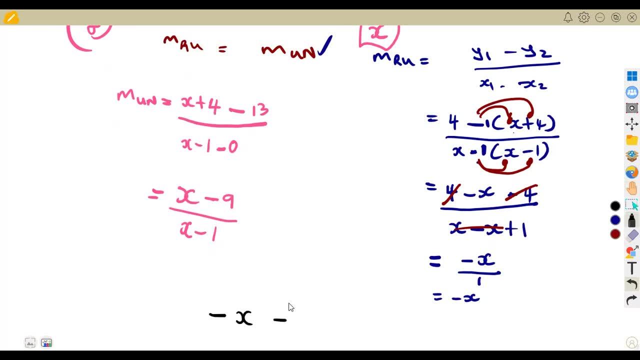 So you're going to have the gradient of RRU, the gradient of RRU which is negative X. So it means that the gradient of RRU, which is minus X, must be equal to the gradient of UN. All right, So this is the gradient of RRU, which is equal to the gradient of. 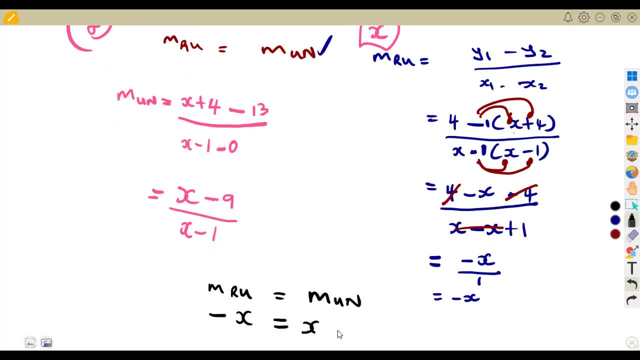 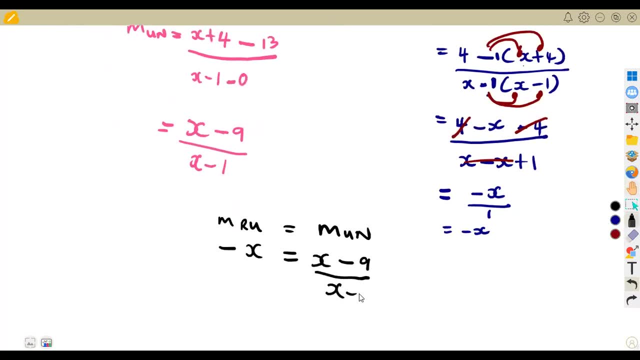 One. What of UN? and UN is X minus nine over what over X minus one? Okay, So, like I said, this can be written as over one. So you formed, uh, an equation. It is having a fraction, We are having a fraction there and we want to solve for X. 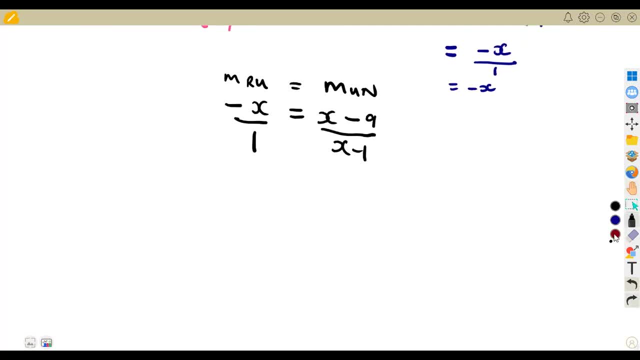 So from this concept of our gradient, the gradient of this line is equal to the gradient of the other line. So it means here We can just find, uh, the value of X by cross multiplying, since it's now an equation. So the minus X here is going to multiply everything in the denominator here. 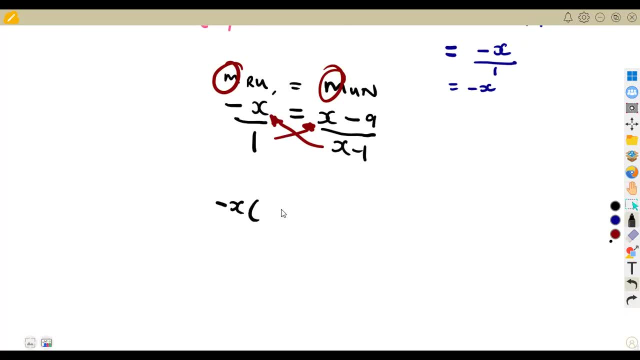 So it's going to be minus X into X minus one, just so that we can properly multiply everything. Then one is going to multiply everybody, As you know, guys. one times anything. it remains as it is. one times five. it remains as five one times six. six remains as six one times seven. 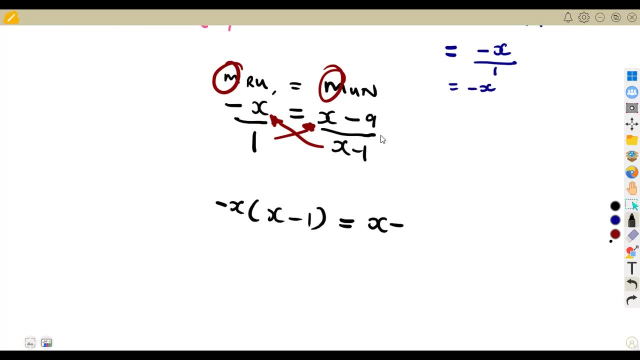 So If you multiply one times X minus three, it's just going to remain as X minus four. one times X minus nine, It is just going to remain as what? as X minus nine. So these, we can expand the brackets on the left hand side. 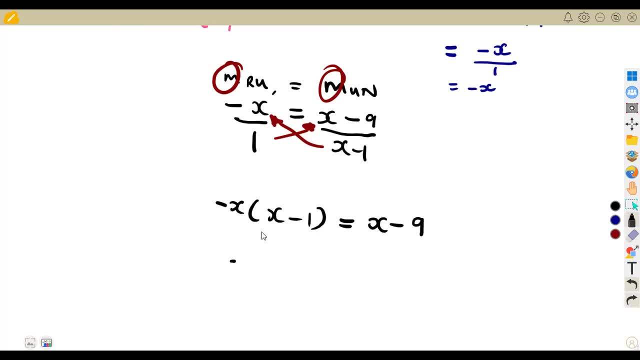 So that's minus X times X, which is going to give us minus X, squared, minus X times minus one, That is going to give us a positive X minus minus. Okay, Then we transpose the X to this side, but you can just write first X. 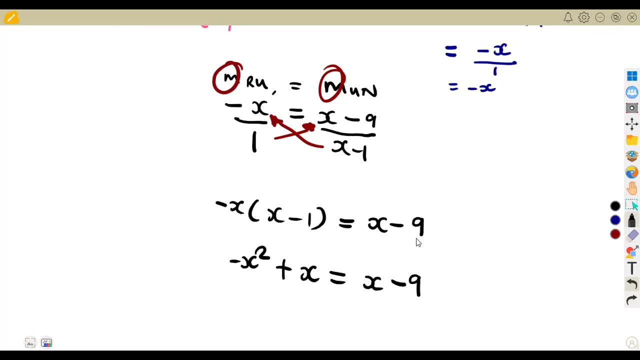 Minus nine. before that. All right, We were supposed to have a normal quadratic equation because, as you can see, the highest exponent that we have here it's a what X squared. So we're supposed to take all these terms to one side of the equation so that we have AX squared plus BX, plus C is equal to zero. 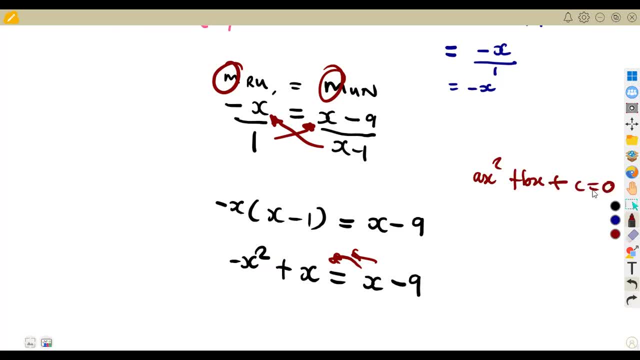 Remember our format of the quadratic equation: plus C is equal to zero. So if this is the format that we are supposed to have, therefore, let us transpose these terms so that It will be minus X squared plus X. the moment I transpose these X to the other side, it becomes a negative X. 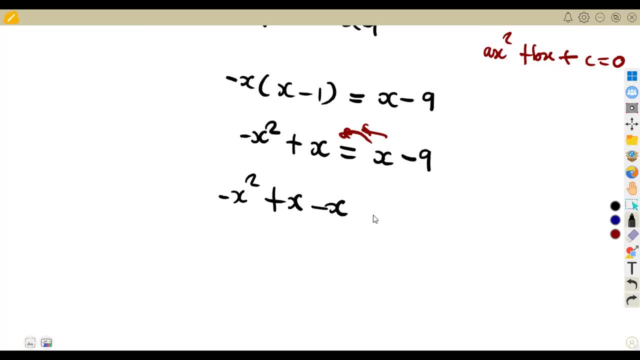 So that was going to be minus X, minus nine. to this side, It becomes a positive, So that will be positive. nine in this case is equal to zero. All right, There's something happening here. X minus X gives us a zero. This is one X. 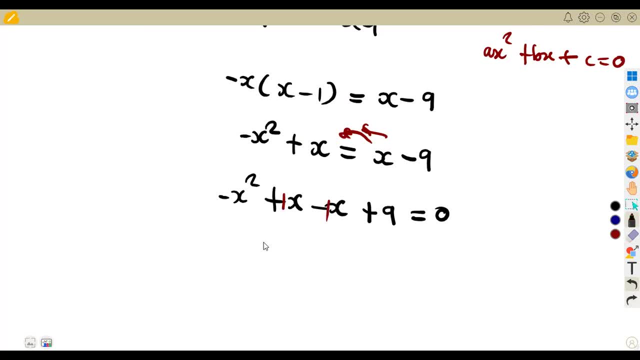 This is minus one X, So it means one minus one, That's a zero. So you're going to have minus X squared plus nine, which is equal to zero, Which is a Three times what two square. So to avoid errors, depending how you can solve was it's still a quadratic region that we see. 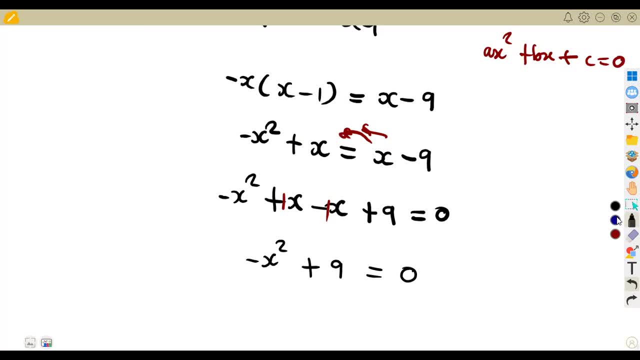 But we know that We can have it in the form that we remain with X squared is equal to a certain term, so that we can introduce What the Square. so how can we do that? Let us just transpose negative nine back to that side, guys. or we can just transpose the explain, because we can be like 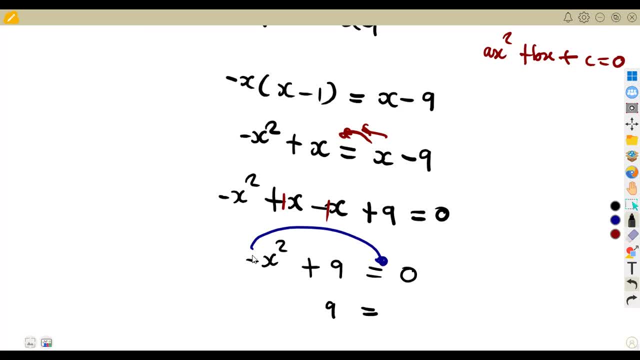 You're playing around this time, All right. So 9 is equal to. because negative. yeah, we want this to be a positive, so you're going to take it to the, to the other side of the equation. so it will be positive x squared. so as long these two are, 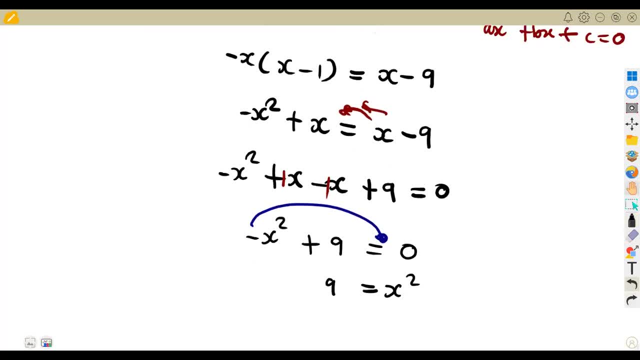 equal. guys, it is the same. it's the same thing as x squared is equal. do not be scared, okay, it's the same thing. x squared is equal 9, it's just one and the same thing. all right, 9 is equal to x squared. x squared is equal to 9. it's just one and the same thing. it's either. you're going to introduce the. 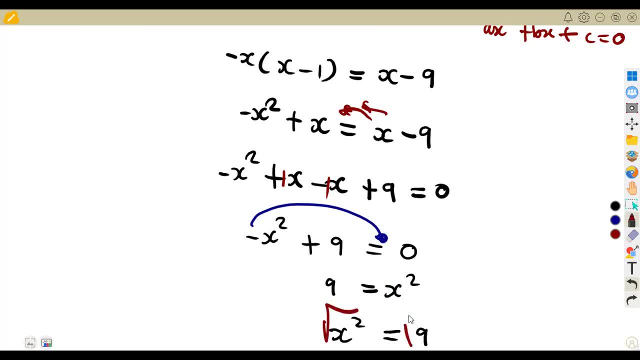 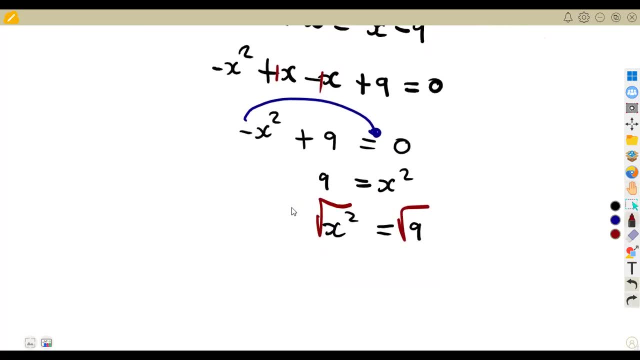 square root here or you're going to introduce the square root in this way, which is one and the same thing. so what is what matters is that we want to remove the square, the square. the opposite of that- to remove this square is the square root. so the moment i introduce the square root here, it